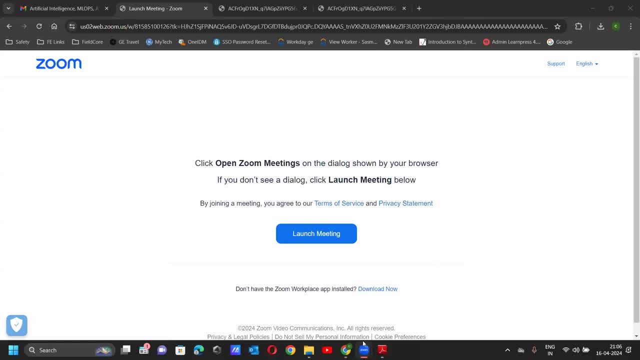 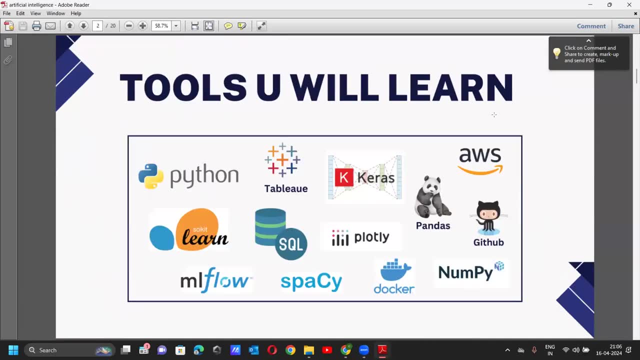 to share with The project details. I am just adding The syllabus. I think it's whatever is there same thing, but the project details that we have discussed, right. So syllabus, in the sense you will be learning all of this: Python basics, followed by Python advanced, and then all of these. 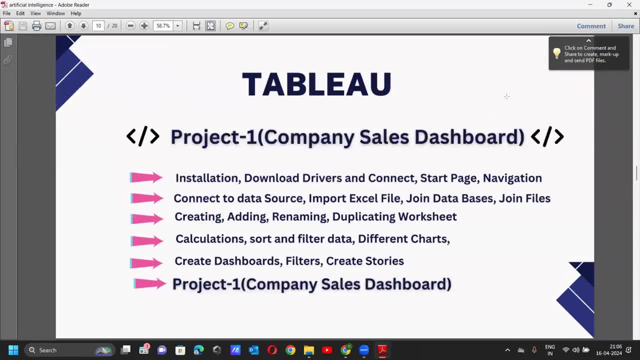 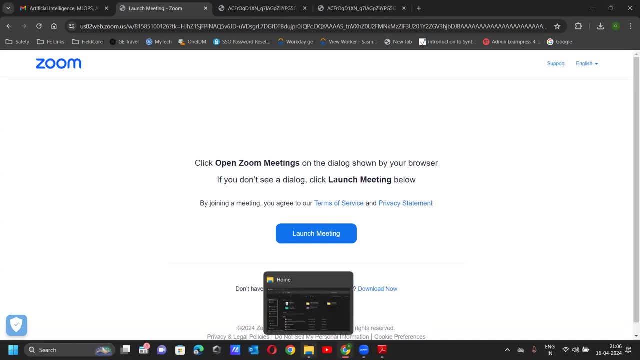 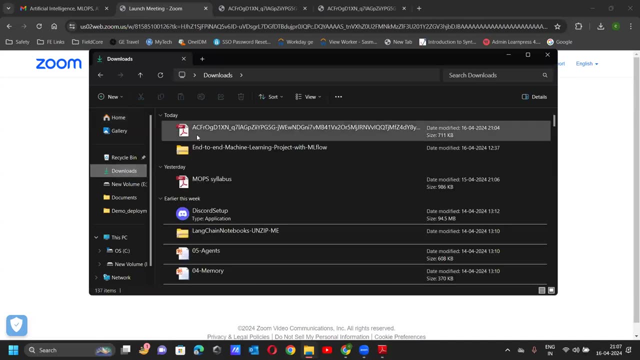 topics you can go through Machine learning, regression statistics, all of these things we will learn, But after that we will be doing projects right? So the project part- I did not get time to complete it. Maybe by tomorrow I can share it with you. I think it's half prepared. 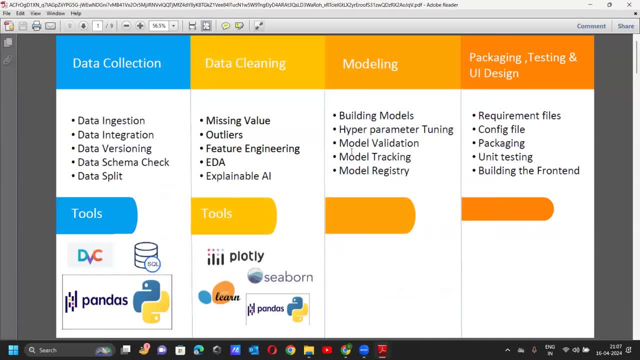 But I think you can get an overall idea. what I'm trying to do here is Every project. I'm trying to create this kind of pattern where you will see all the process that we are going to follow in every project. So, as I said, there will be three projects and every project will be different. 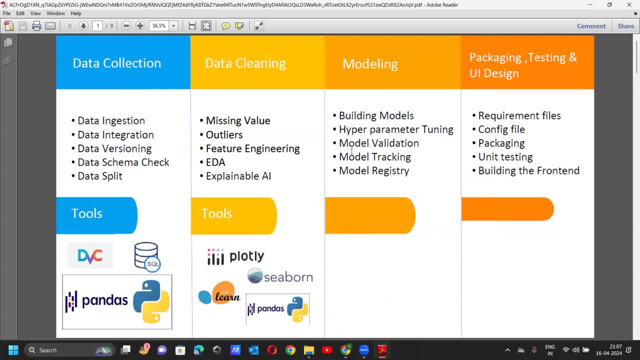 right. For example, the first project is supervised machine learning- Semi-structured data project. The second project will be deep learning NLP based project. So the steps will also be different, Like in the second project, in the data cleaning it will not be. 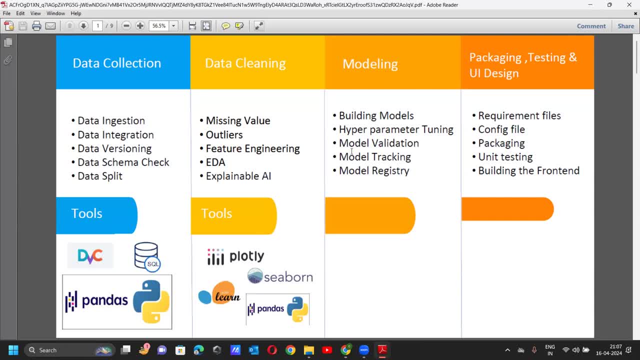 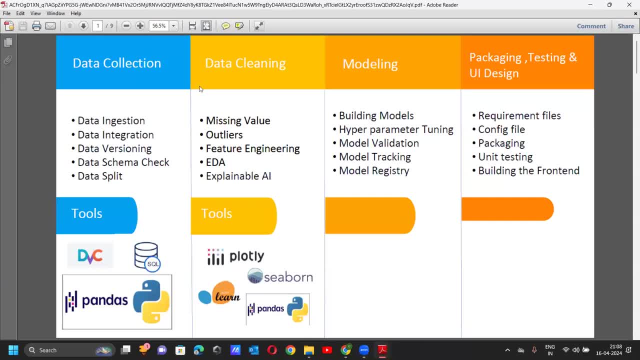 And for the first project, the first thing is data collection. So what we are going to do is we're going to data ingestion, data integration, data versioning, schema check, data split. So all of these things we will be doing in the first step And let's say, the data is present. 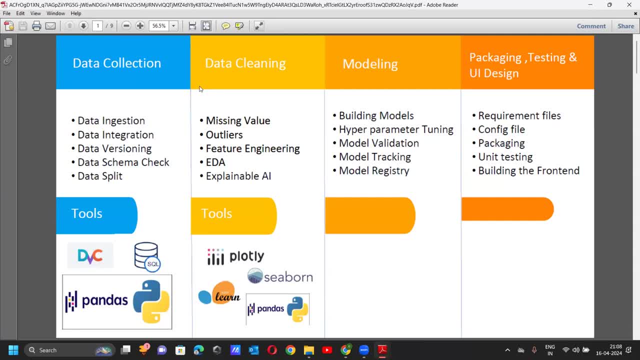 in three different places. One is in SQL table, So we need to write a script which will go to SQL and collect the data from the table and load it into a data frame. And another thing is we need to write a script which will go to SQL and collect the data from the table and load it into a data frame. 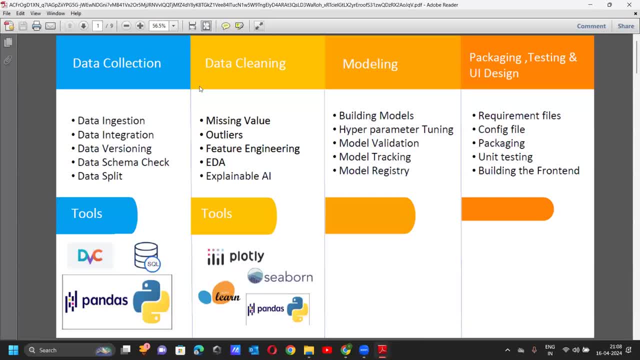 And another thing is we need to write a script which will go to SQL and collect the data from the table video. And another thing is we need to write a script which will go to SQL and collect the data from the table and load it into a data frame And so you can get the data local and then we also have the data. 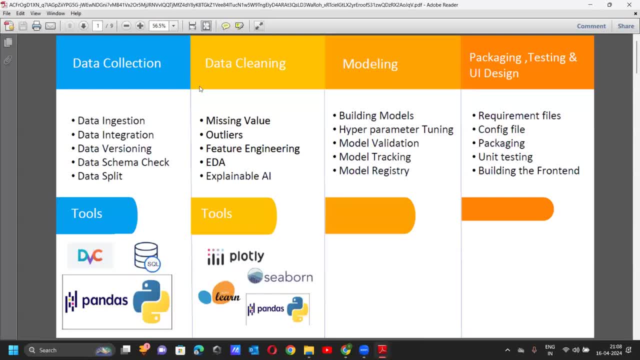 collection. so we no longer need. we as a cloud, you can copy the data and after the data, let's say it's a CSV file. And then let's say we have one more data which is present in MongoDB. So we have to write three scripts, basically connection script, That is, data injection, After the data. 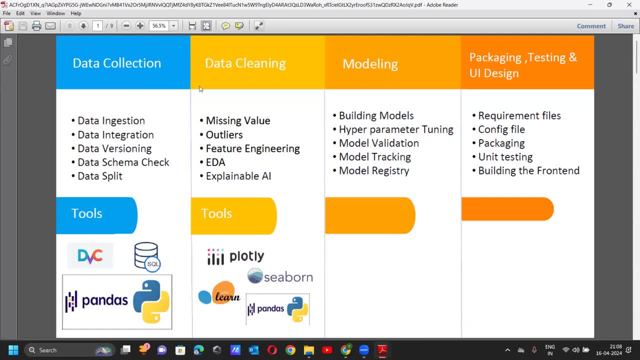 integration. So we need to basically combine all of these three data frames into one so that we can do our processing on it. Data reconciliation means whatever count is there before and after loading should be same. So we'll be writing three, four scripts basically in data collection. 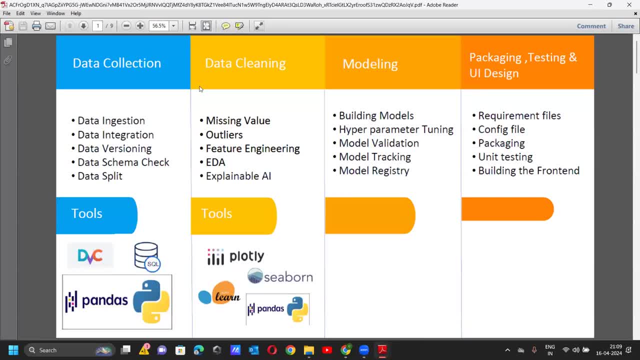 part. One script will do data ingestion. One script will do data integration, And let's say it's a continuous integration and continuous development. So it's all automated. So today your client has given you something, but what if the table has modified, has been modified by the? 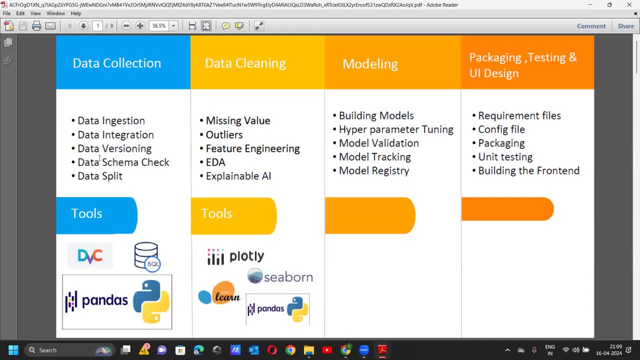 team members, right, The data engineering team members? or what if the data has changed from the source So that you can check from data versioning? So we are going to use a tool called DVC, data version control And using that we will able to understand if there is any change in. 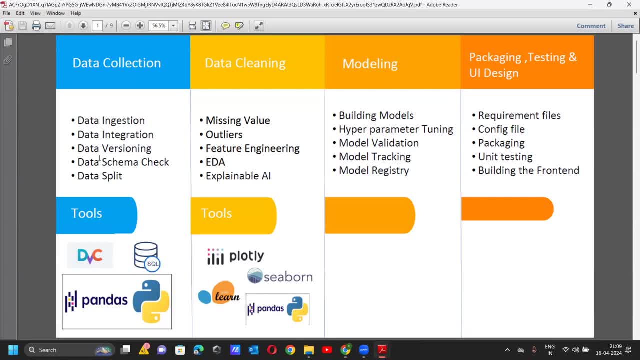 the source right, So it will show you like it's like Git, So you can see if any modification happened from the source. Schema check So we can also add test cases Like we want, certain for example. let's say we have a column called cells and all cells value should be number. 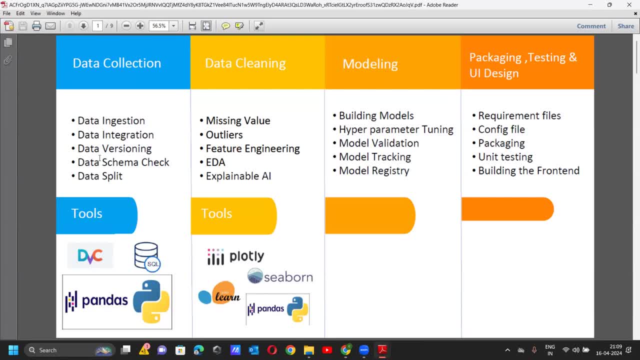 Sometimes people write dollar Also right, Like the, let's say $1 million, So dollars. I mean it should not be string It is, it should be strictly integer. So those kinds of schema we will be applying, And so you in in a 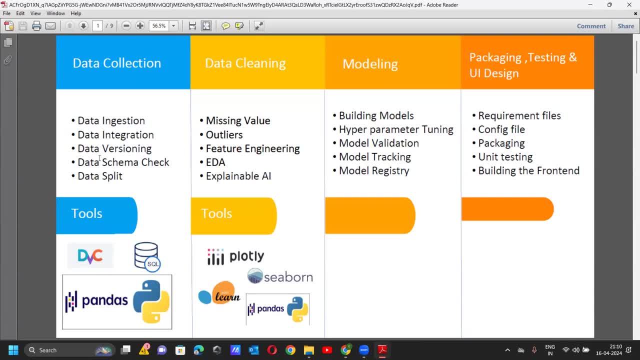 high level at a high level. So it's all about data collection, right. So different sources and then data integration, data reconciliation, versioning and all that. So we're going to use SQL, MongoDB, Pandas, Python, DVC for the first step. Second step is cleaning. So once you have your 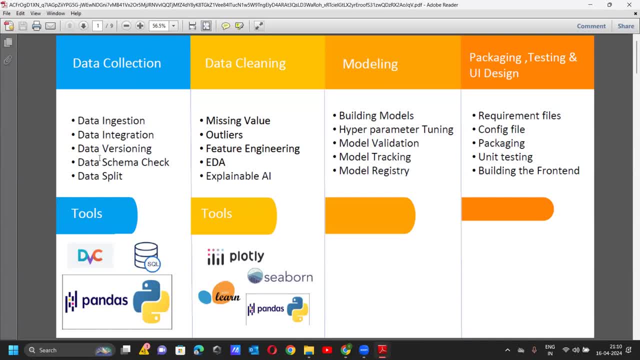 data. you will be reading your data like missing values, outlayer, feature engineering. EDM is exploratory data analysis or visualization, and explainable AI. So these all steps are my own steps. You will not find it from internet anywhere, So I'm thinking every step and writing. 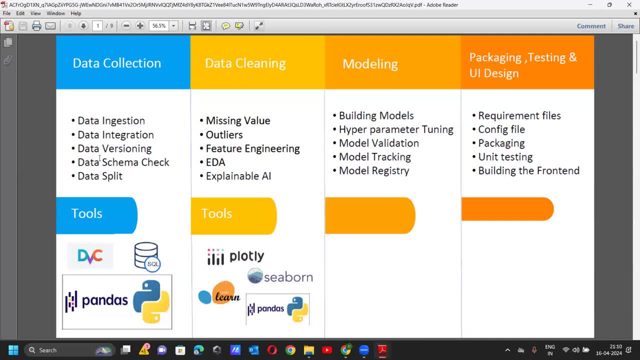 So it is taking some time right. So for explainable AI you can use SAP. you can use a lot of model interpretable libraries from Python. for outlayers You can use a scale on. for EDA visualization You can use 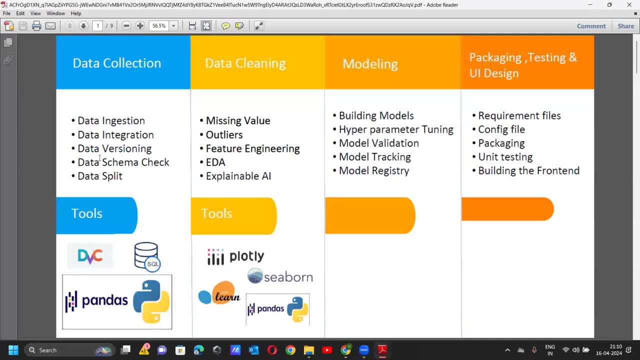 Kotlin and Seaborn right For missing value you can use Panda. So all of this cleaning, once you have done that is again another script and that script has individual package. So one package will do, um, basically missing value treatment, One will do outlayer, one will go feature selection. 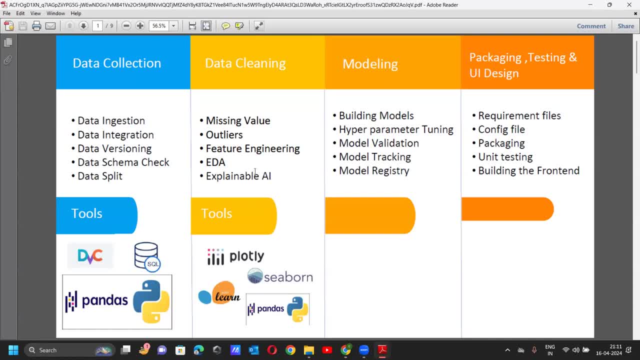 We'll create pipeline. I'm not written yet, but now it is coming to my mind. So that's called data pipeline creation. So one after one after one after. so I will just write: the uh flow, right. 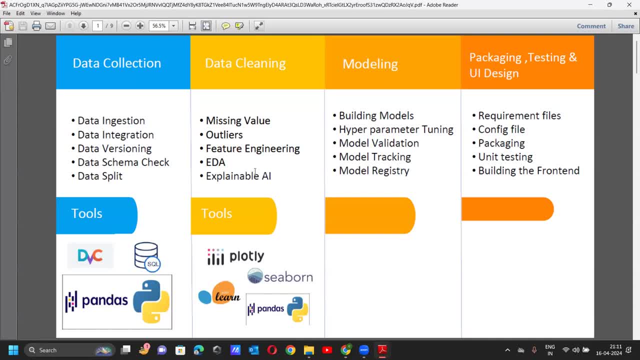 First You do this and then do that, do that. So one one one I will call and create the pipeline script. So this is the data cleaning. After that we'll go for modeling. So in the modeling, basically we'll. 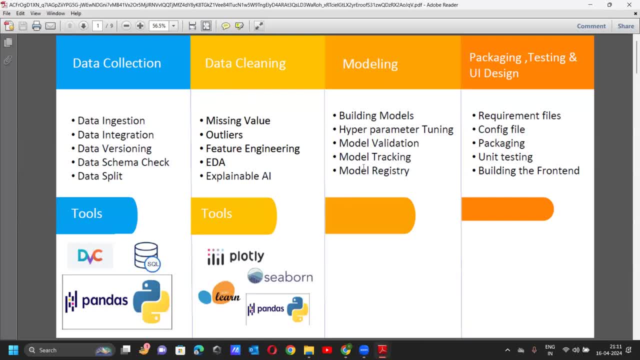 be using machine learning, And here I will be explaining you all the algorithm of machine learning related to the project. Uh, it's not like step one we will be completing. No, we have a lot of things in modeling. Also, we need to try different algorithms. uh, four, five, six, seven. 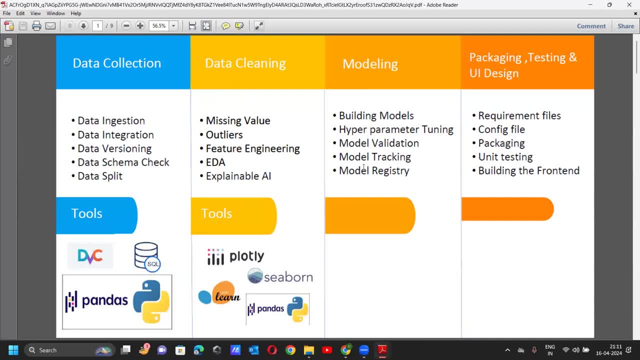 how many algorithms? right, For every algorithm we need to do hyper parameter tuning, So we need to do that And uh it it is like every hyper parameter tuning we do It's called experiment. And uh, when we have a lot of algorithm, it is really chaos, Like you manually cannot track it. 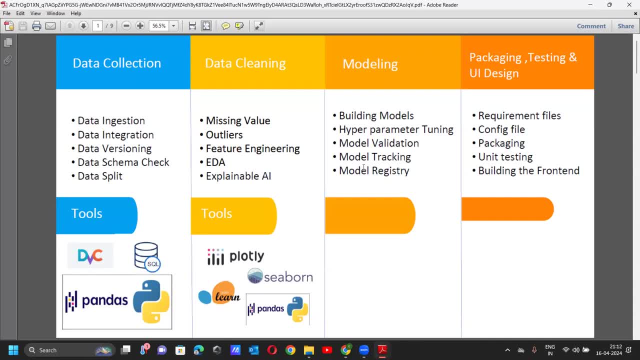 So we'll use ML flow for modeling. So we will uh use model tracking and model registry right Uh for ML. uh, from ML flow we will build our model, We will do hyper parameter tuning, We will validate our model, We will track our model and we will register our model. That is a step. So every 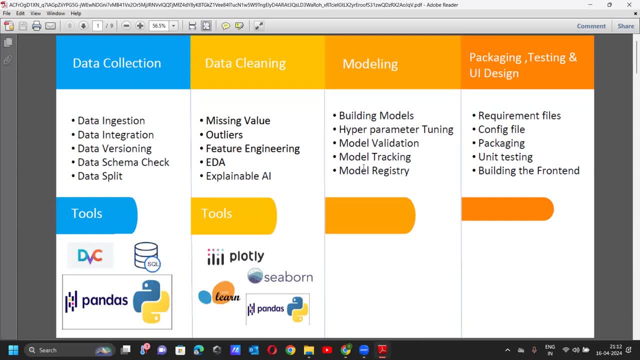 step is a step. We will edit a simple script. We will keep our script. You can see how many scripts are in there, right? Um, you know, every script is a step. So if you're learning how to run a model, you can apply the model. you can apply the model. You can buy a product or you can. 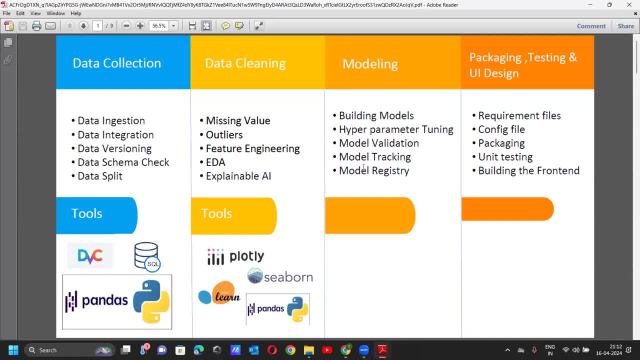 buy a product, or you can buy a product whatever. So we're going to start with three, four, three, four script. So you can understand, one project may have 15, 20 scripts in total, right, Um, I mean. 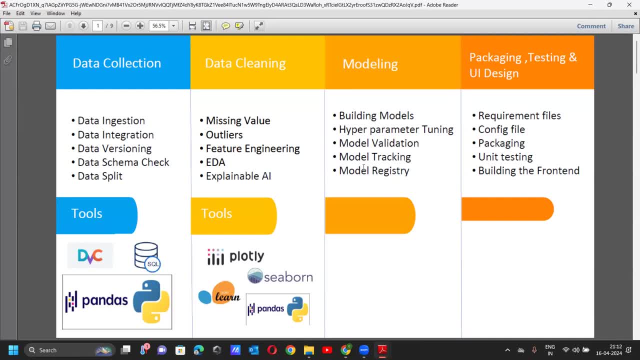 now data collection, we have two, three scripts. data cleaning will have maybe feature engineering, one script EDA, one script outlay, missing value, maybe one script explainable. AI may be another script. So three, four scripts. modeling: You may have two scripts, one for building and one for hyper. 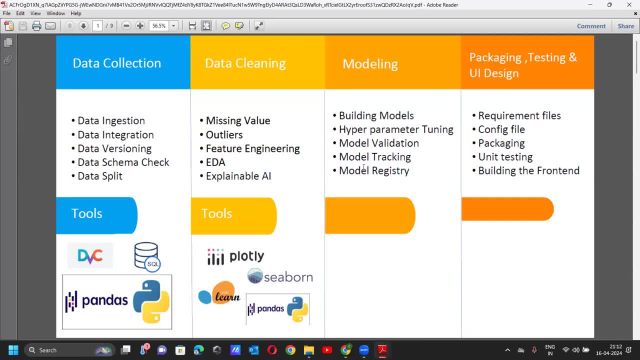 and ui design. so once we do this, we will go for a config file, so we'll mention all the configuration and everything. we will package it, unit testing. so, as i given you one small example, the schema check, we will do a lot of things. we can write our test cases using pi test. we will do unit testing. 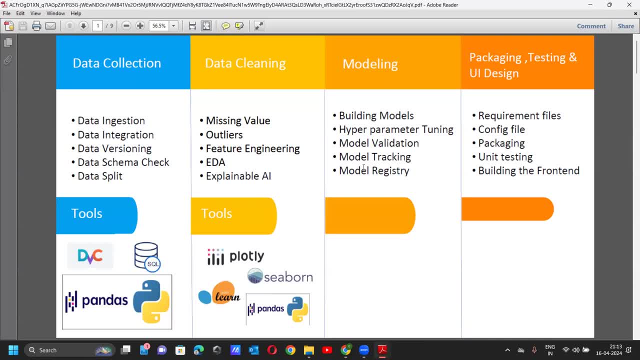 once everything is done- bundling and packaging, everything is done for this. also, we are using ml flow and dvc combined right for packaging, so we have something called ml model and ml package. right project, ml project- sorry, in ml flow, so which will help us for packaging- and pi test for testing. 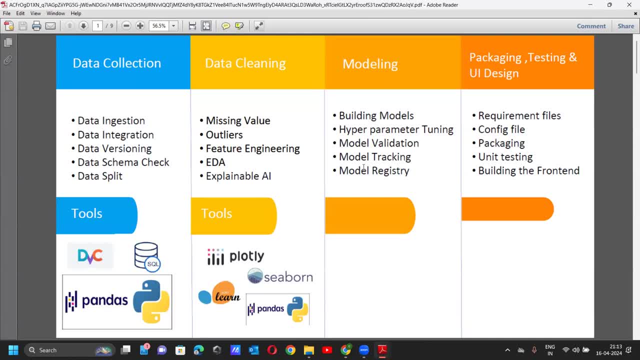 so, once everything is done, we're going to build the front-end part. front-end means the user can upload data and the user can get the predictions right. the front-end page, we'll build it using streamlit. i have not written the tools. the idea is, for every step, what all tools we're going to use. i will write it. 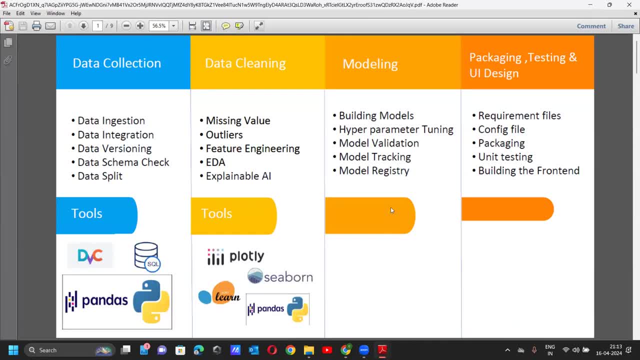 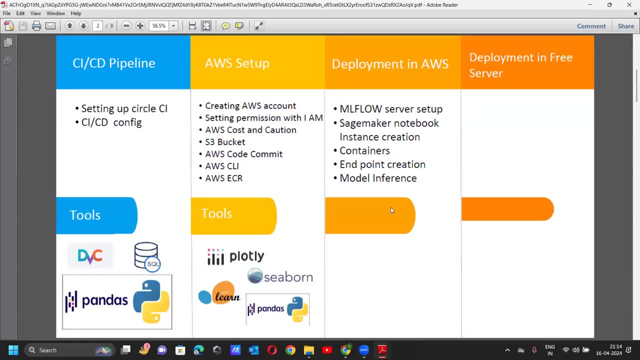 i have not completed. maybe tomorrow i can show you. but in the packaging we'll be using streamlit. after that we'll go for cicd pipeline. so i have a lot of options. i was thinking which one to use. i think github action is the best one. so we'll be using github actions to create workflows and in a 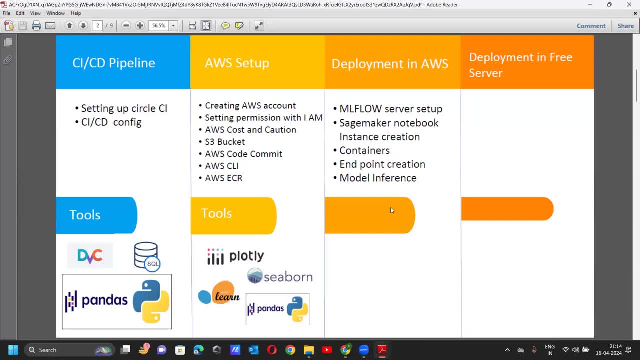 way, we will be automating our cicd pipeline right in the next step. and after we do this, we will jump into aw s, we'll do some setup, we'll create our aws account, we'll set our budget. otherwise, when i was a fresher, i was just like i forgot to set budget and the bill was like three, four thousand, right, so you. 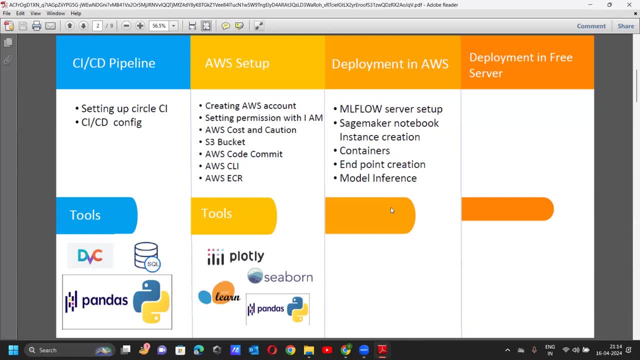 have to be a little um, uh like, little uh conscious, right. so when you're using aws, most of most of the things are not free, so you have to set your account permission and then i am user all of this s3 bucket, commit, aws, clr, ecr. all of this setup we will do. once the setup is done, we will go and because 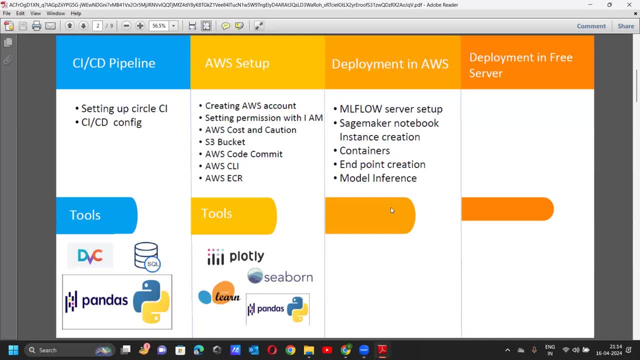 after cicd pipeline: our model is done like everything is uh completed. we have packaged it, we build the front end, everything, uh, we have created the pipelines for cleaning, modeling, validation, everything is done, then we'll go for deployment. so once so far, whatever we have seen, it's local. we will go to ec2 and create our ml flow server setup. after that we'll go to sagemecha. 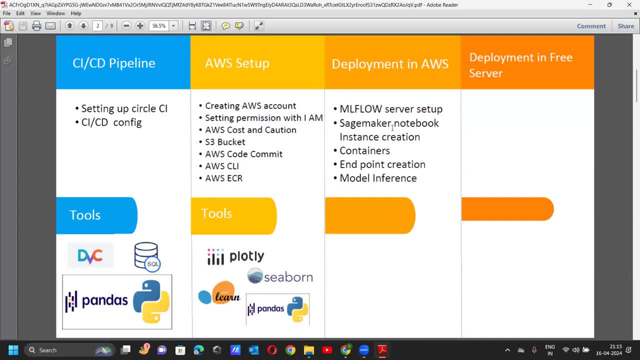 create notebook instance. we'll containerize whatever we have created the image. we will push it to ecr, elastic container registry. so after pushing the image, we'll create endpoint and then model inference. so once we have done this, our model will be deployed in aws. you can get a url. 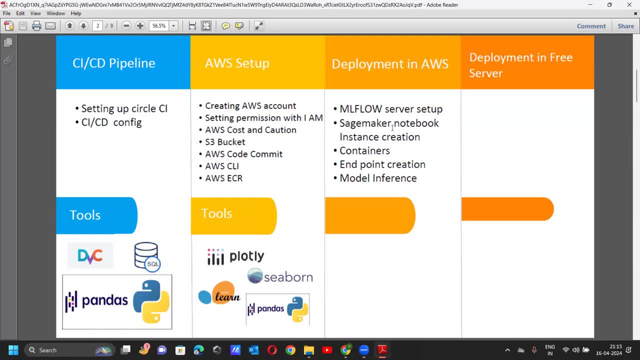 and from that url, universal url, so you can upload your data and you can see the results. right. so here the project ends. uh, also, at the last step, i will show you how to deploy it in free server. i will be using very small data set. i mean for local. i will be using real data, but when we go to 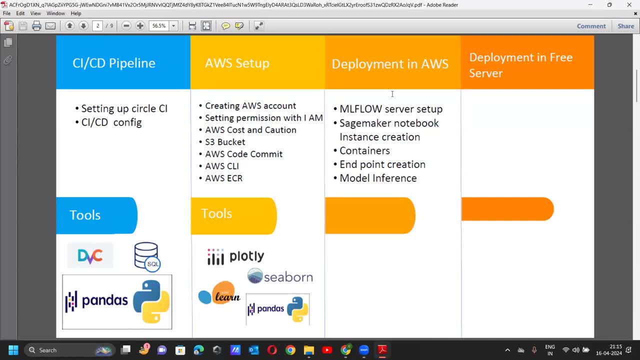 deployment in aws. it's just the process. you should know why you will, because when you run ml flow, lot of experiment will be generated and it will take space and memory. so i'll be using a very small data set just to show you the deployment part and the small data set we will also use for 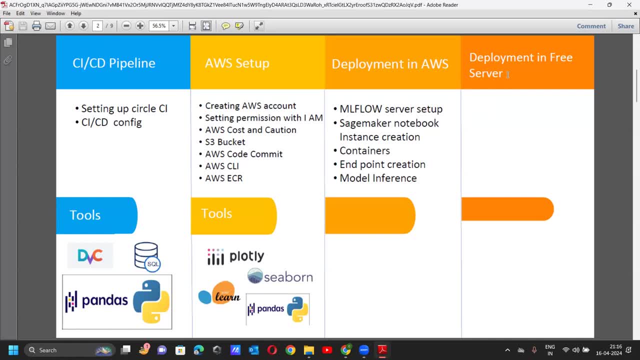 deployment in render. so it is a free server you can deploy and you can get a url, this url or heroku, any platform we will deploy, and this is for your portfolio. building this you cannot always, uh, keep it up and running. it will cost you, right, it's not free, so this just for. 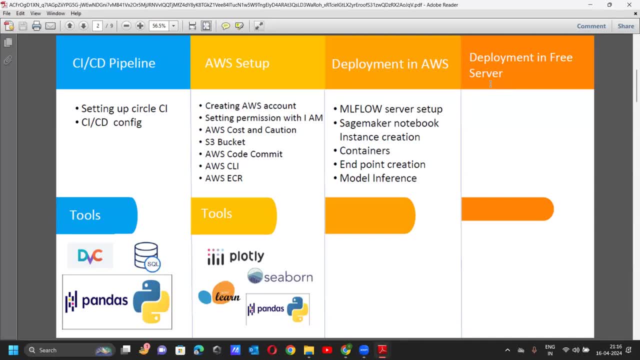 your knowledge. but this last part is for your portfolio, so it will always be up and running and you can create your digital resume where you can share this url, like what you have built, the github code along with that, uh, this particular server. so this is a complete project and we are going to iterate this process for three times. 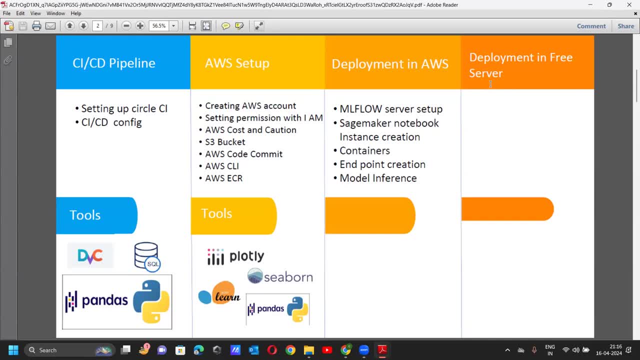 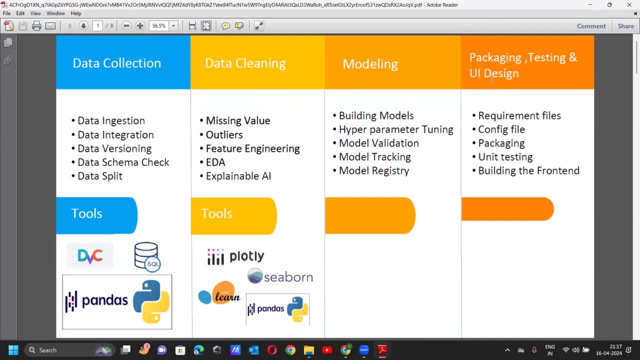 for every project. the most of the process will be same, but some processes are different. for example, in the second project, data cleaning is completely different. modeling is completely different. packaging is also completely different, why? because it is text data and deep learning. so modeling, we will be using deep learning, hyper parameter tuning. here we will use escalon, there. 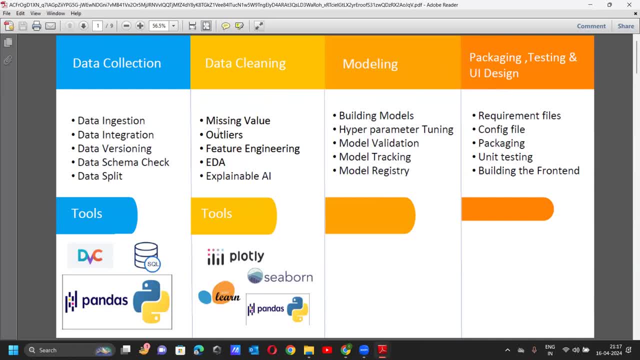 we will use tensorflow or keras, um and uh. missing value out layers are not there in text data, so we have um stopper removal embedding, different kind of uh cleaning and data injection, also different. here it is semi-structure, but that is uh text data, right uh? so it will be in pdf format, so we have different code for the initial. 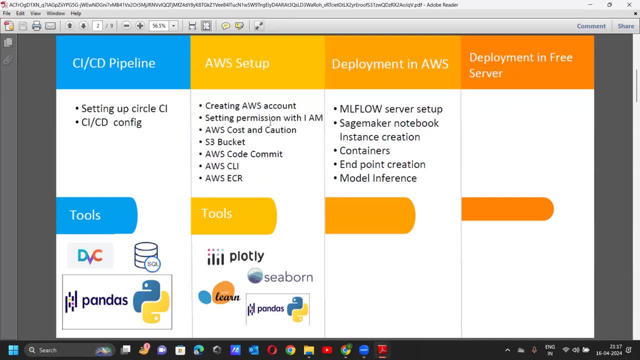 three, four, but i think in fact in the second project also, cicd, aws and deployment is almost same, right, uh, i think these are same, but the first four will be will be different from project to project. so i think you got an idea, so we will do this. but before we jump into 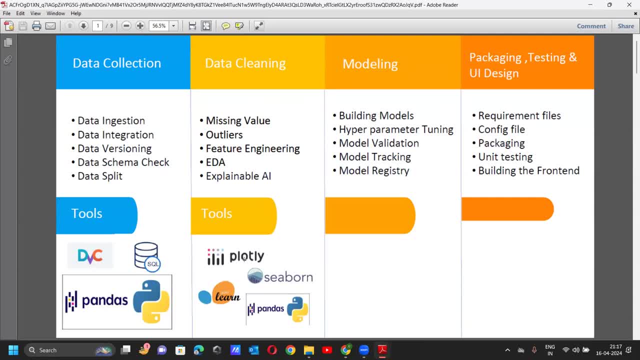 this mode we need to have some basic understanding. you can see here i'm using plotly seaborn escalon pandas, so if you don't know these libraries you'll feel very uncomfortable when we go to project initial few days i will be teaching you the fundamental libraries which are required to 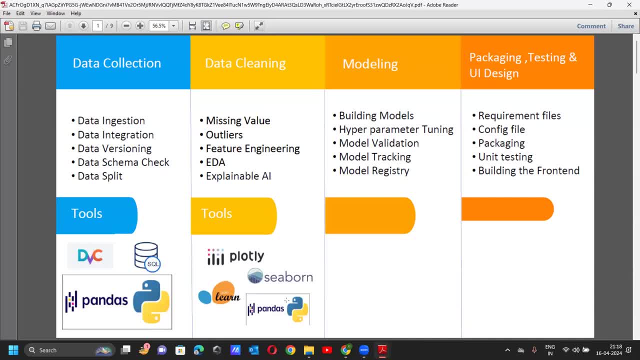 build the project. uh like pandas, like plotly, right streamlet um basic understanding and statistics, machine learning theory, algorithms, everything we will understand and then we will jump into project. so the whole course is project based. so if you ask me, where is machine learning here? all are like ml ops. so, as i said in the initial, like 60 or 50 of the time. so don't worry. 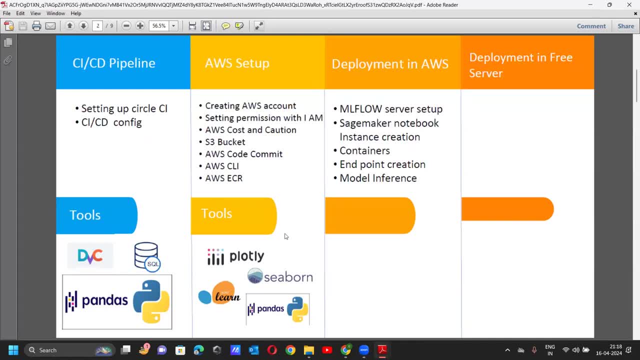 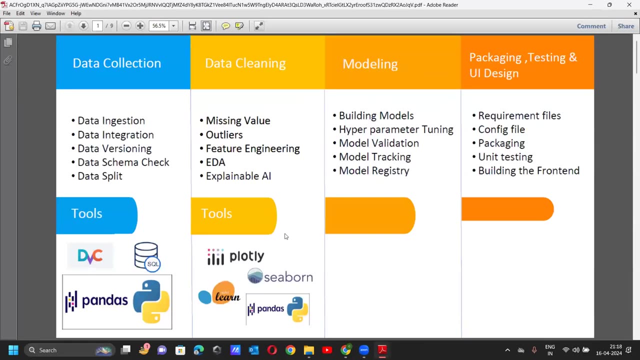 about the last four things: cicd, aws, setup, deployment, uh and free server. it will take time for the first project, as i said. second, third project: most of the time thing is same, so you can very easily- i mean quickly- within hours you can do it. data collection, cleaning, modeling is the major task which will take time, cleaning especially. 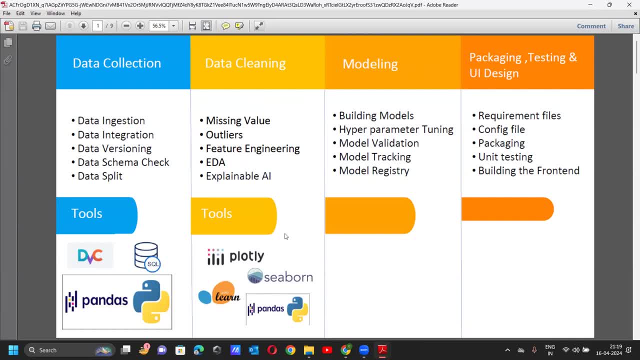 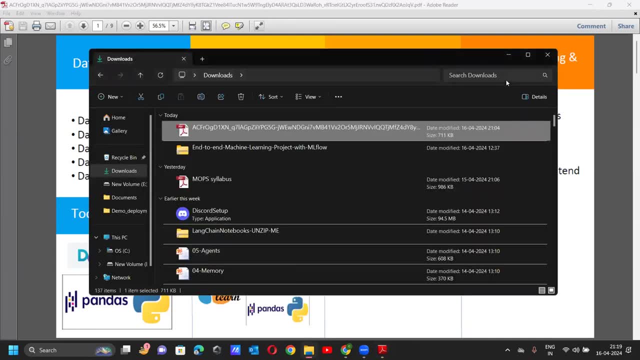 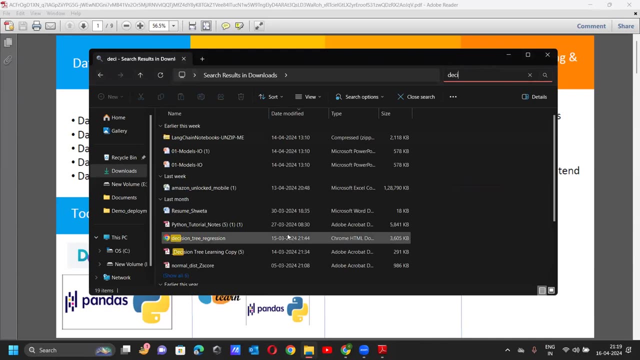 cleaning will take a lot of time. and modeling: when we go for modeling without algorithm details, we will not go there. all the algorithms in detail way we will discuss. for example, let's say i'm talking about, let's say, decision tree. okay, today i'm going to implement decision tree, so i'll be showing you. 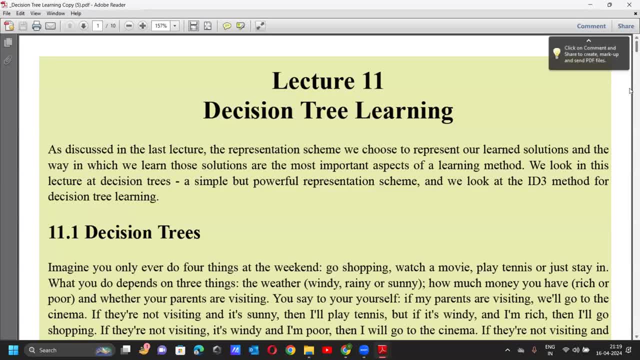 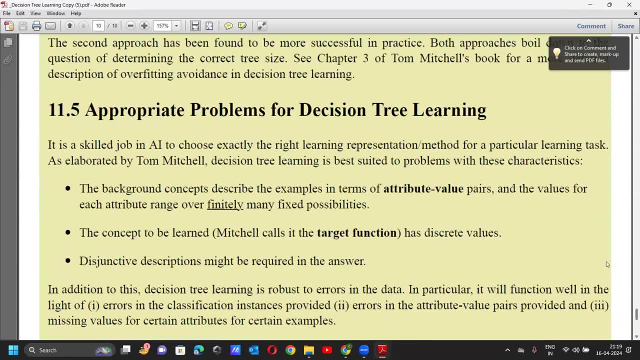 how to use decision tree algorithm. first i will explain you- this is the note for a decision tree- i'll explain you the theory, um right, complete theory- and then we will go and we will deploy right. so once you understood the theory, then only we will go for coding. 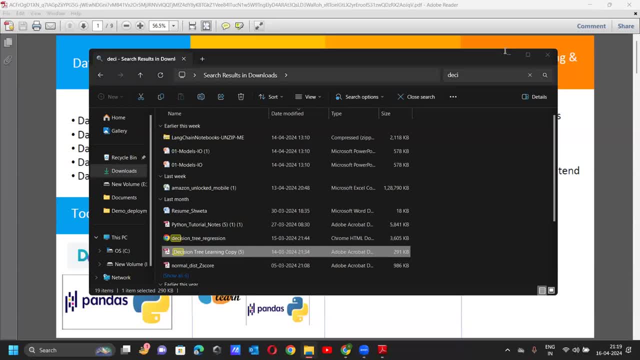 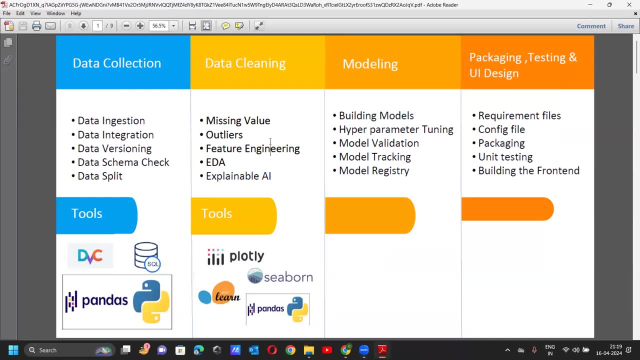 that's how we will do, and this tag that you are looking here will vary from person to person. i think there is not a single tool. right same task can be done using multiple tools, for example, model tracking, registry, validation. all of these things can also be done using ml, run ml flow, so a 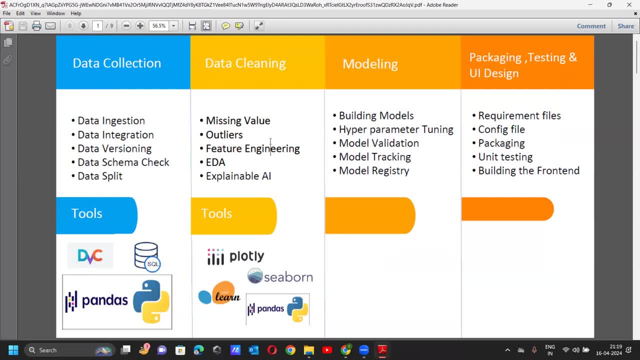 lot of tools are there: gen, ml, different tools for ui design you can use stimulate, flask, dash different. so i am picking the things which are very popular. uh, having said that, there are alternate options are also available. deployment: you can do it in azure or gcp also, but aws age maker is very popular. right ml flow is very popular by because 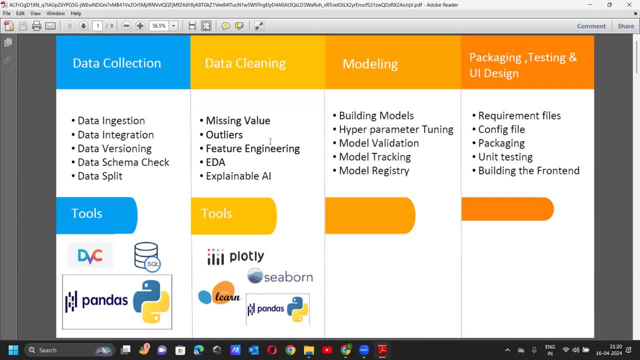 it is by databricks. dvc is very popular for data versioning, right? uh, stimulate is super easy, anyone can use it and quickly you can build. so i think this is all about the project. i think you got an idea at high level. today i have nothing much to share with you. all the questions i have answered. 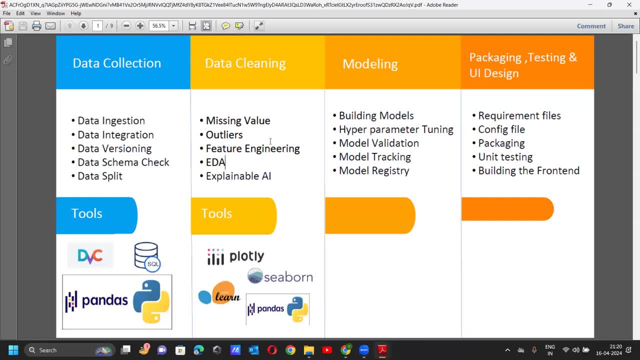 yesterday. um, i will complete this thing for three projects and, in fact, project detail also. i can share with you what projects we will be doing and we will be also understanding the architecture, like the system design or not system design, but architecture means from where data is coming and 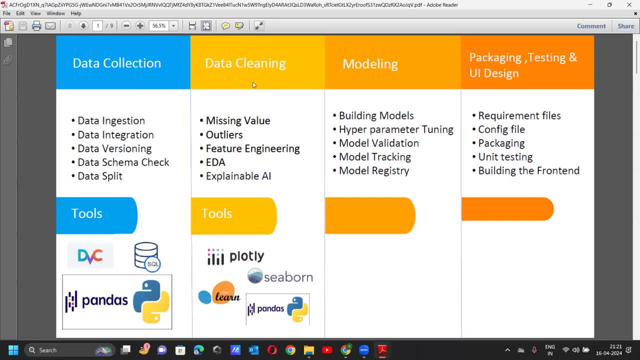 from where it is going. what is the entire flow of data? so like this you need to repeat. so three projects i'm doing here and three more categories, different categories. if you complete for every project, i think you are, you are okay, like you can handle any kind of real-time problem, right. 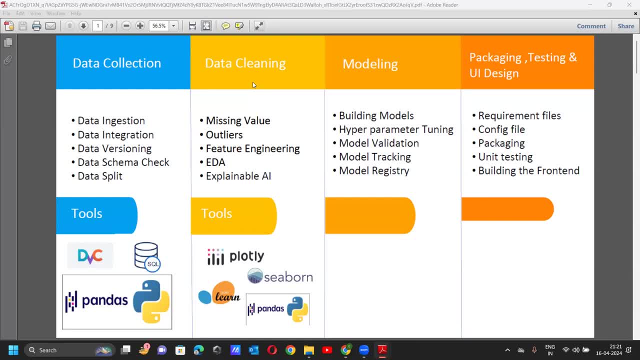 any question with respect to this. data mining is a different and different data mining. data cleaning is okay. so when we are talking about data science project life cycle, these are the steps: data collection, data cleaning, modeling, deployment, modeling, validation, deployment and monitoring. right monitoring is also important, so data cleaning is a major. i will say 60- 70 of the time. 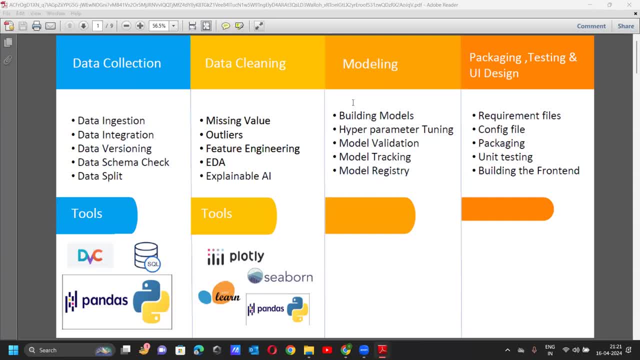 you will be utilizing in data cleaning, and data cleaning is very different from project to project. every project data cleaning you will see different, like in this project, regression project. that's why i have written these steps. if it is a classification project, i might not be uh worrying so much about. 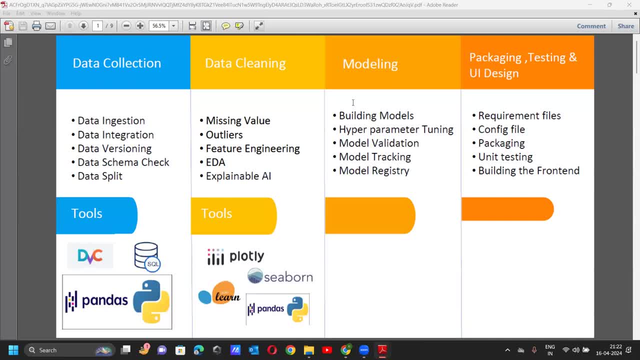 let's say outliers, if i'm using tree algorithms, maybe i will be adding class imbalance, different kind of problems, right? if it is a text data, i mean stop word removal- embedding different kind of cleaning. so if it is evaluating, so cleaning will vary from project to project. depending on your data, cleaning will vary. 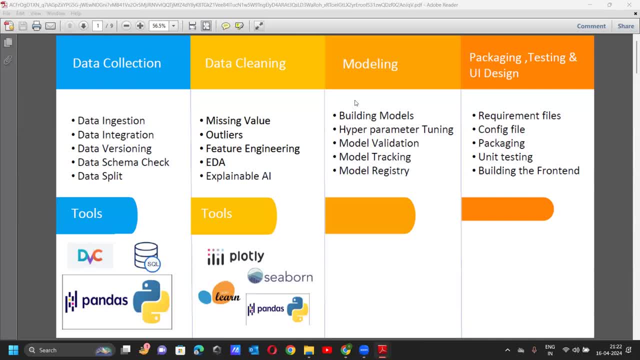 modeling. again, i think this is also automated. so once you have done this, for one project, same script, you can reuse 80 percent of the script. you can use, in fact, this project packaging testing ui design also, mostly, yes, ui design. obviously it will vary from project to project, but requirement: config: packaging: same folder. you just need to change. 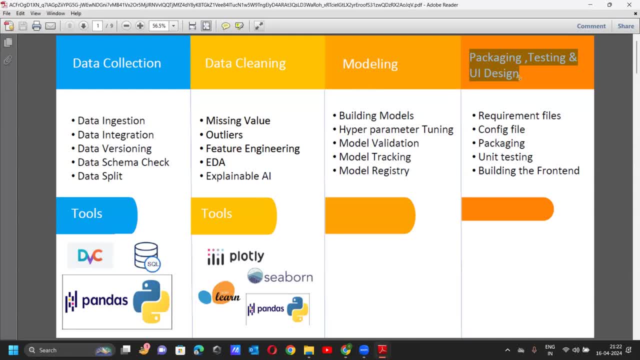 little bit here and there. so once you have done the first project, 80, 70 of the code you can reuse. if it is not text and deep learning, i think if it is classification project, 80 you can reuse. but if it is a big data project, obviously everything will different. 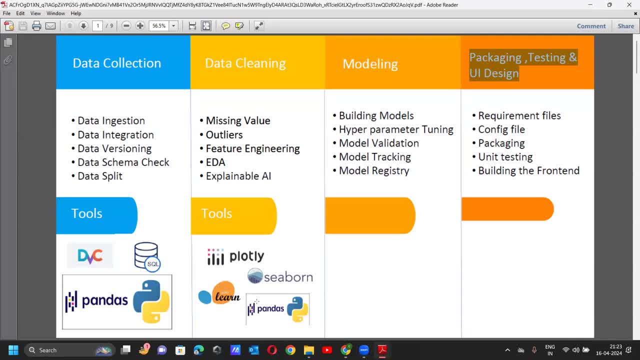 right, you will not be using pandas, you will be using spark sql. you will not be using sklearn, you will be using spark ml. so entire project flow, steps are same, steps are same, but the approach, the tools that you will use is different. right, okay, yeah, yeah, yeah, yeah, yeah. i just have one question. 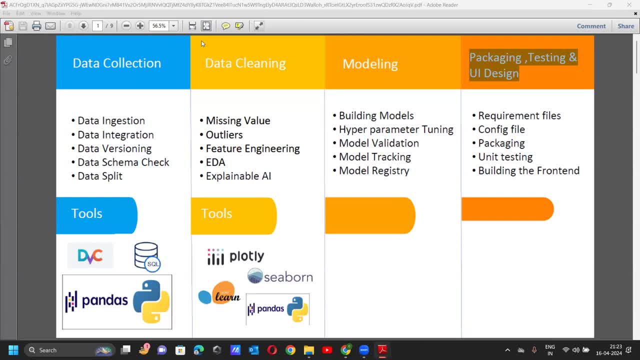 uh, actually i have six years of experience, but uh, mostly in the networking, okay. so actually i have a background of program. i mean i know the c language, okay. so uh, by taking this course right, i mean, after how many months can i start uh giving interviews like 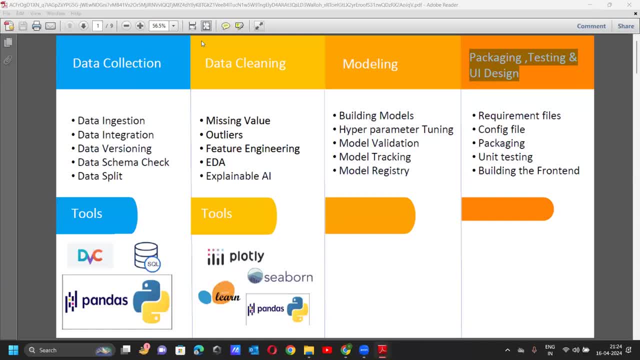 we can. you can start giving interview, maybe after we finish first project. first project so you can say: at least you will have some, not some, but at least you will understand the flow. uh, after one month i think you can start applying, but once you complete the course and 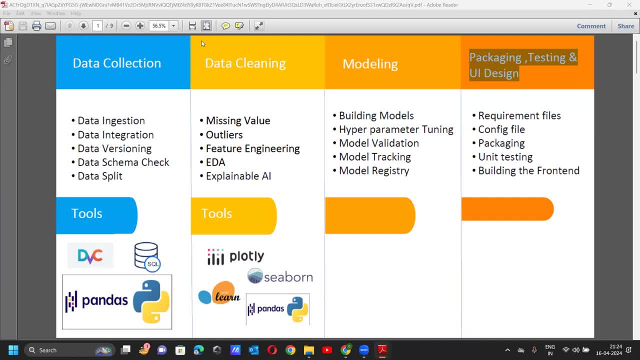 revise it once, you will get a lot of confidence. uh, you can start applying after one month. yeah, one month, or one and a half month? okay, so considering right, i mean how many? so you're saying two to three years, we can claim right, or anything smart enough you can claim. see, it's all depends on if you know the park. 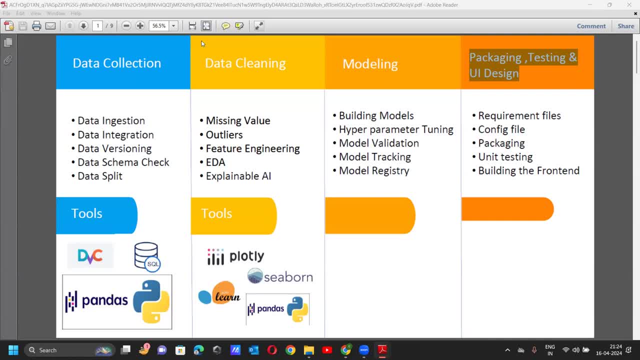 what i said is in in data science, there are seven to eight different templates. right, this is one template for supervised semi-structure. so every template, if you complete, you can showcase: uh, five years. also senior data scientist, you can justify. having said that, i i will not recommend to do that because in data science, because it's a new field, 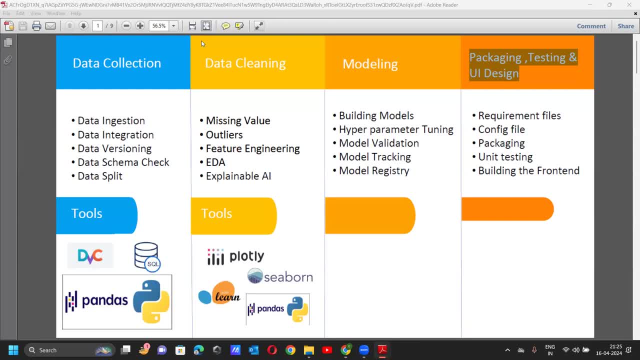 uh, five, six year experience means it's not a data science, because in data science, because it's a new field, uh, five, six year experience makes you have a chance to do it for 5-6 years or even 30 years. it is a lot of pressure on you, even if you are selecting in the in the role. uh, i think, uh the. 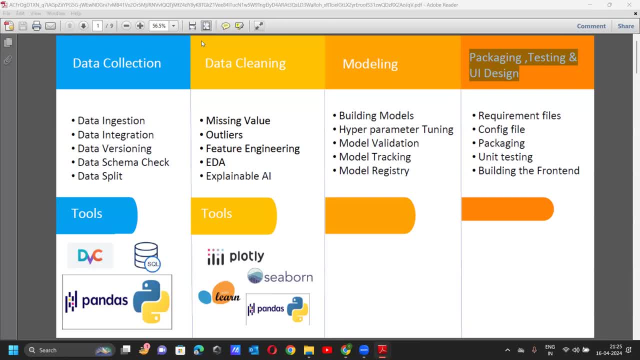 expectation is little more. um, it all depends on you. i cannot say, but this course is in the safer mode. if you want to ask me in the safer side, i think um two, two to three years. i'm saying if you are smart you can justify three, four years also, because you have. you know the pattern now. 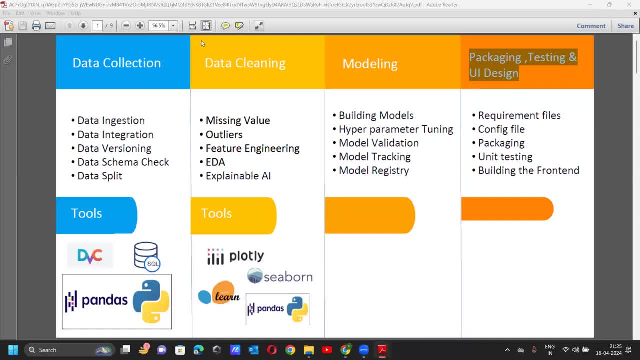 you learn spark and same thing you implement using spark. so that is one pattern. see, when you go more and more experience means what they will ask you: variety and uh uh. fresher means you might not be knowing a lot of. i mean, you might not be knowing how to handle text data. you might not be. 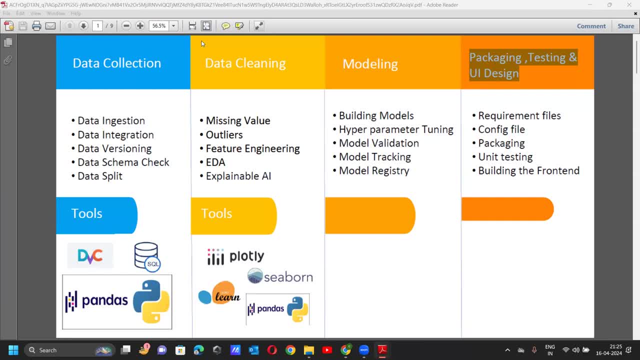 knowing how to handle uh- deep learning related, uh- image processing data- right, but if you are senior, senior and senior, you will get a lot more project experience, and that's what is expected from from senior data scientist. so there are three major roles: data scientist, senior data scientist, lead data scientist. 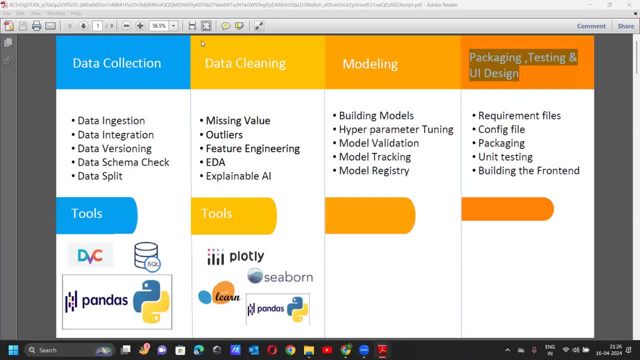 uh data scientist means fresher. uh senior data scientist means a person who, who has uh very good knowledge in different, different kind of data they can handle, like big data, small data, image data, text data. at least they should know. they might be expert in one, but they should know other things at least. 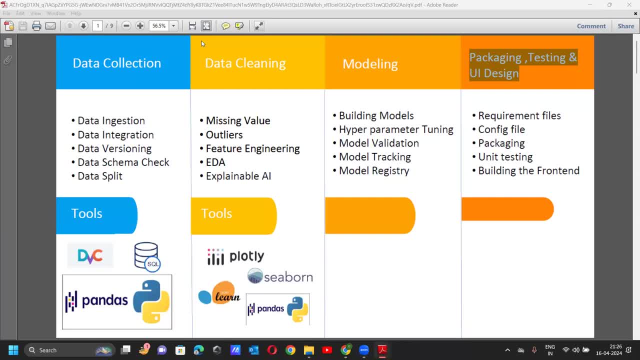 one, one project they have done. they have some basic understanding. that is senior lead means you will be individual contributor and as well as you will be generating ideas, means what many of the client- many of the time the client- will not be sure. you will look at their data and you will give solution. what else you can do for them? 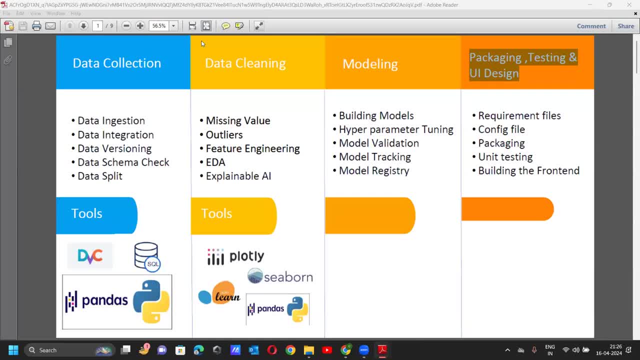 everything. so you are a person who will generate project for juniors. yeah, yeah, i mean i don't have any. i mean i don't want to mention more than two years of relevant experience, but yeah, so after this course, i can apply only for data science roles, right, or any data in list, or i can. can i apply for? 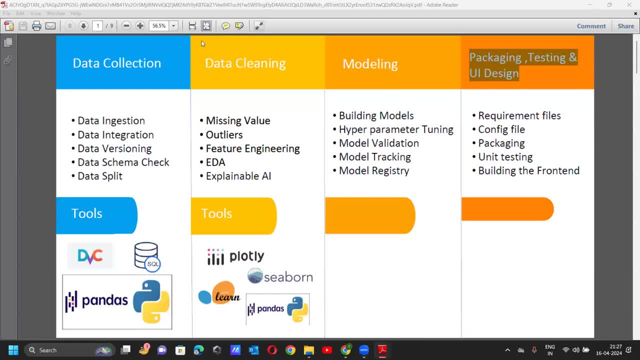 those roles as well: data analyst and, uh, those kind of roles. just give me one minute, yeah, yeah, yeah, a data analyst, uh, data analyst, you see? i mean, um, yeah, you can apply for data analyst power bi, you can learn along with this right for data analyst. i think the visualization is very 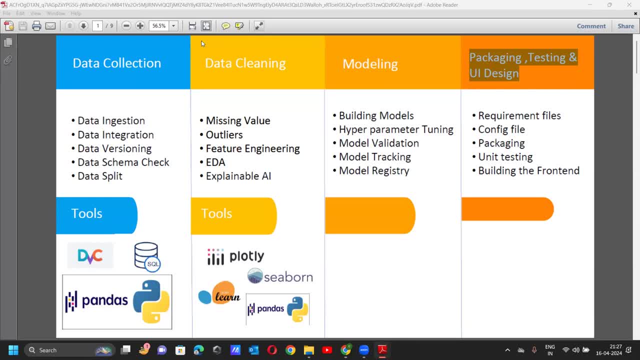 important. so many of the companies they use power bi along. yeah, i mean you know plotly and all that, that's fine, but mostly business analyst. data analyst means you should know one bi tool. so power bi, if you learn. uh, this is an advanced code, so all the data scientists are data analysts, right? 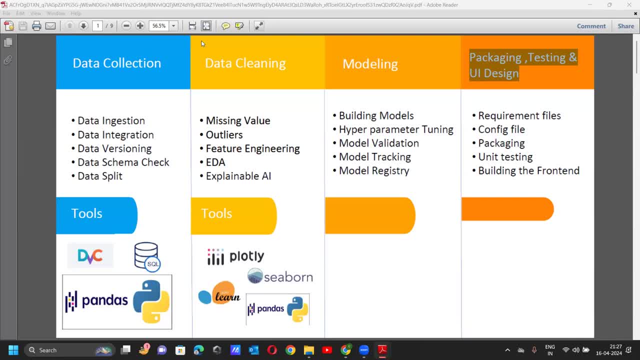 are you waiting? data analysts are half data scientists. all data scientists are already data analyst. so i mean, if you are hearing, this course means you are eligible to apply data analyst, mlops, data science full stack. but one thing is missing: power bi. you have to learn yourself and 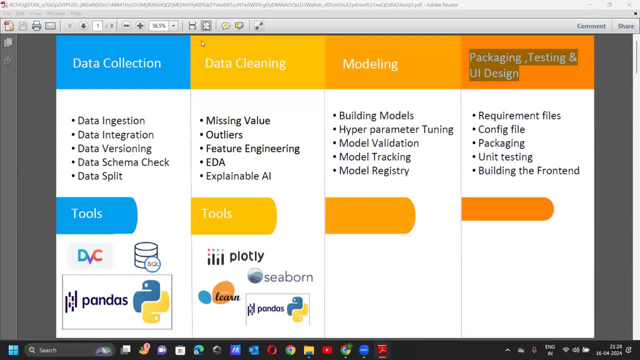 big data is universal, so everyone should learn. along with big data, you should learn power bi, okay, so, like i have one final question, so as when i see in the industry- right, i mean mostly people will start with uh and data analyst and after four or five years of experience, right, they move into. 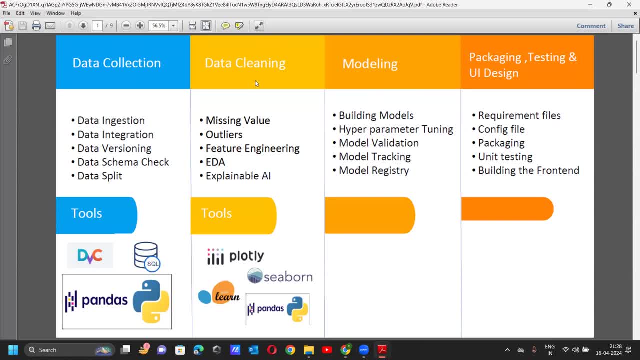 data scientists, i mean as per my company. so do you recommend going that way or, you know, straight away going to uh data scientist roles? like according to me, according to my prediction, you will not see data analyst role in future. it is going to be absolute right, like in uh- current i mean you- you may find roles. 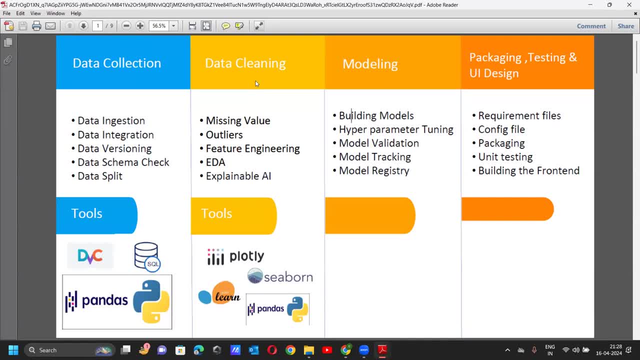 available presently, but it is, even if you are getting rose, very less role will be available and there's a high probability that will be layoff. a layoff will be very, very, very much in why? because data analyst job, mostly descriptive analytics they do. descriptive means what you have- historical data and creating an like you are generating insights from the 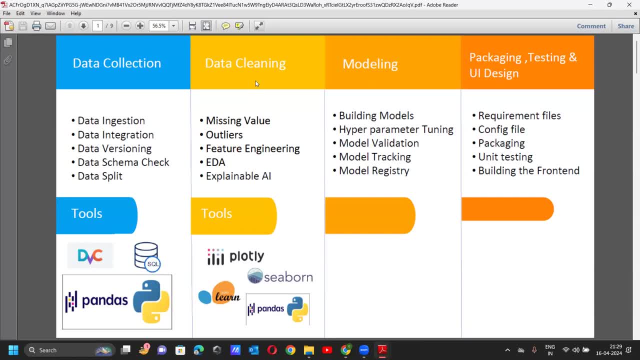 historical data. data scientist means: yes, they will do predictive. sorry, descriptive as well as predictive means what? obviously historical data analysis you will do, like this is the eda. you are doing explainable ai, so feature engineering, so this is anyway descriptive, but predictive modeling, so you're also doing predictive right. so if you can do everything, why they will? keep only data analysis, and i understand, i think, that, as you mentioned, leadこれubeq, you're not gonna get good level of data analysis because when you start as a definer in in part of uh, you're a linear surgeon, you're always very Opera god, so, like i had a good but button. so so are you a data scientist then? um, but how do you think, like you really care how men are the? 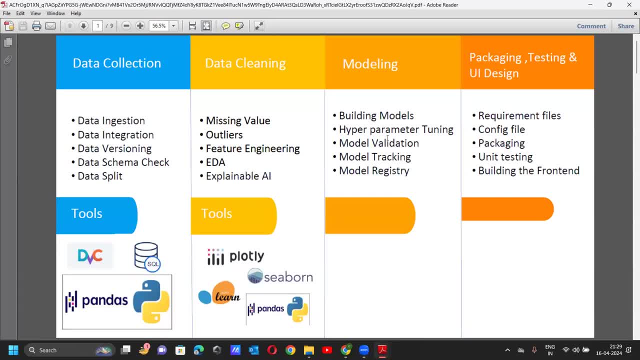 and we are having tools like chart, gpt, llms, which can code right and you have. i think there is some uh. there are some security issues. maybe that's why companies are not adapting, but i think in future that will be solved. so there is something called uh vision, right, uh vision model. so you just 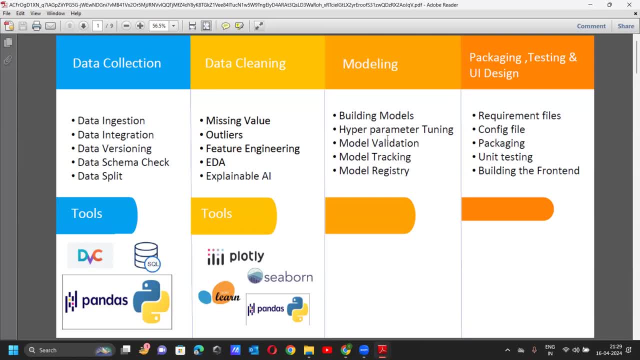 upload your excel file and, like a business analyst, you can ask question, it will give you answer and it can generate report. uh, whatever chart you need, it can generate charts. so a lot of the data analyst job will be automated using ai. so i i believe data only data analyst role, even if it. 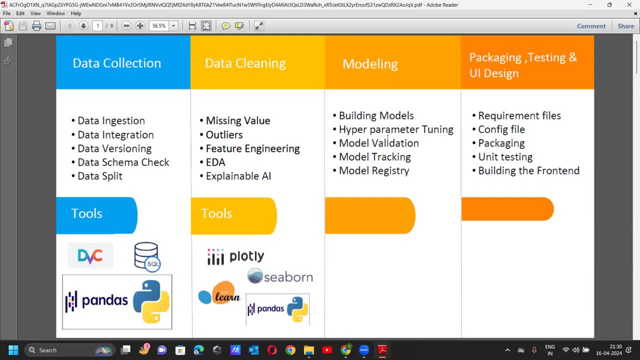 exists, it will be very low pay kind of job it will be. i mean i don't know why such role will exist. first of all because data analyst can be replaceable by ai. ai can do very easily descriptive right. so i mean, if you can target, it was the trend before it was a trend. i mean, if you look at my demos, i was suggesting 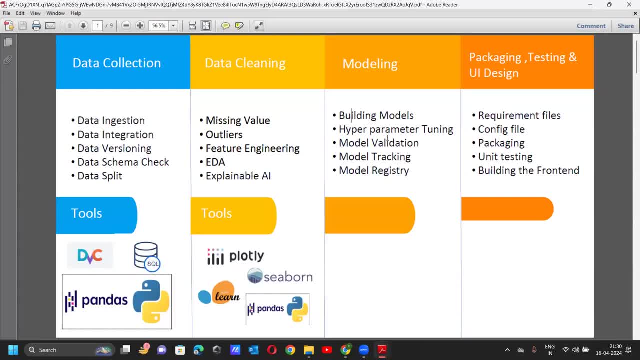 freshers to go with data analyst first and then to switch into data science. but i think now it is because of the advancement in ai right, all of these data roles are getting automated, so now full stack is trending okay. yeah, that's right. yeah, thanks for the clarification. 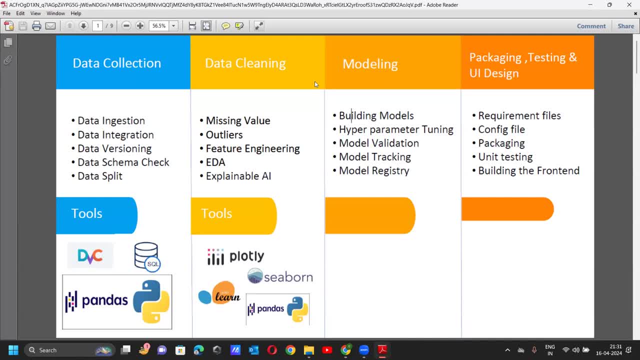 yeah, i mean roles are available now in market. see, many people will say testing is not present. mostly testing jobs are converted to develop development. you must have heard about it right now. it is full stack, a person who is doing development. they can also do testing. but still, testing jobs are. 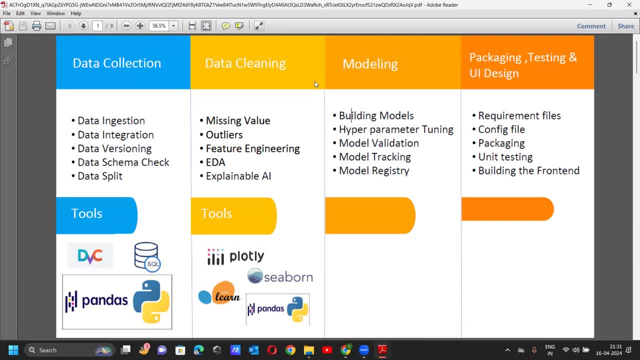 available in market right but less in number. same thing with data analyst. so data analyst, it is present, it may be present in future, but very less uh and uh, most of the people who are doing people who are in data analyst, they will be migrating to full stack data science or data. 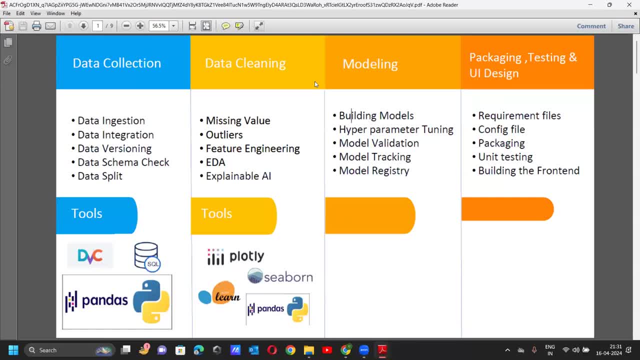 engineering site. right, yeah, i got it. even i saw the news. right, even developing uh language will become english. okay, that is a high level line. so even developers might come to status exactly. so after 15 years i think, if you have seen nvidia ceo interview, so i think after 15 years we will be- 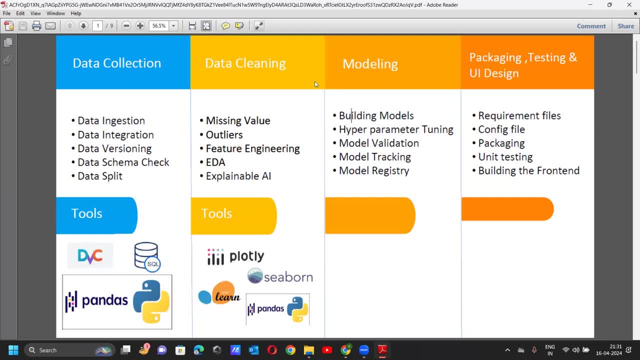 talking to machines using english programming also might not be required. so much so i think it will be a big deal, right? so in those situation- i mean descriptive analytics- it is not a big deal. you just put your data and charts will be created, right, so i think it will be easily automated. so why? 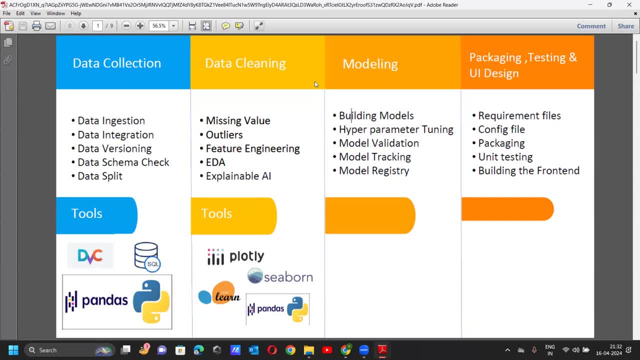 there is a and it is a use case. uh, if you go to startups, they will tell: build llm application which can replace bi engineer like business intelligence engineer or business analyst. yeah, so that's, that's the goal of the companies nowadays. don't go with dataless jobs. yeah, it is, yeah. 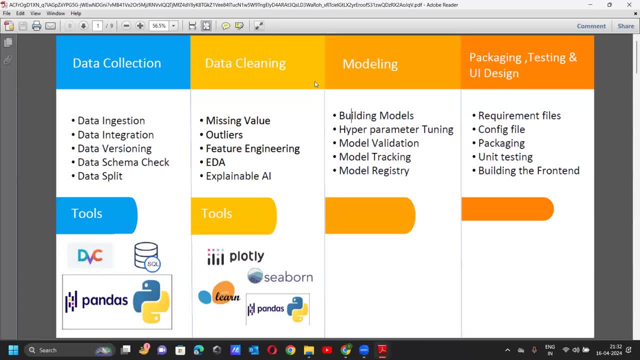 yeah, i got it. yeah, thanks. so, uh, i think uh, that's where we are. so, entire software engineering, i will not uh say it is completely vanished, it will go like it will not be there, something like that, but um, most of the software engineering people. two things will happen. number one is um head count will reduce. that is for 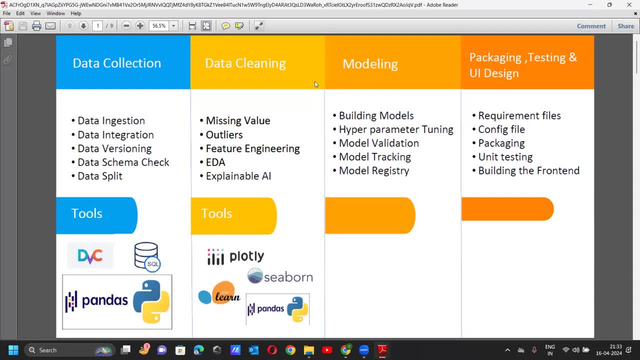 short right? ah, in every domain, impact in ai also, in data science and data engineering also. every field, every field. because of automation, head count will be reduced and everyone will be learning llms, generative ai and this kind of no code ai. no code ai means generative ai, this kind of platforms, right. 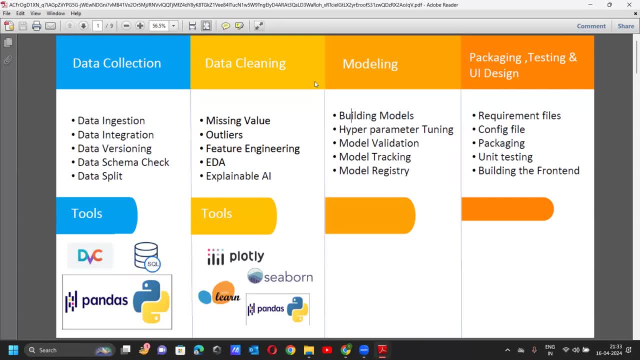 there will be two categories. so all the software engineers will be slowly, slowly, slowly. they will be migrating to ai engineer eventually in next five to ten years, i think the next five to ten years to 10 years, uh, i mean when. when i say software engineering, it is uh, basically ai ops software. 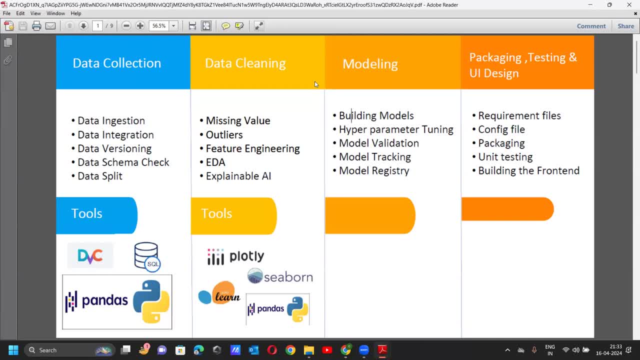 engineering will become ai ops. uh right, most of the things that they are building is ai, only ai, software they will be building and maintaining and there will be new roles which will be evolving, like what? all new roles hardware related. so software is fine, but hardware is also needed. 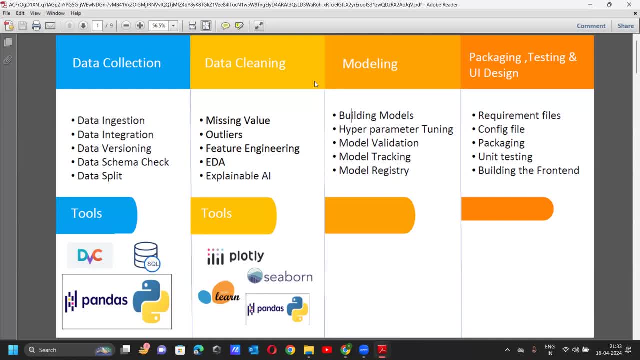 right to build the robot. so a lot of hardware related jobs will open and security related jobs will open. that is my prediction, because a lot of data. who will secure the data and this data? they are training on every data. so who will control? who will uh uh, who will do that security? 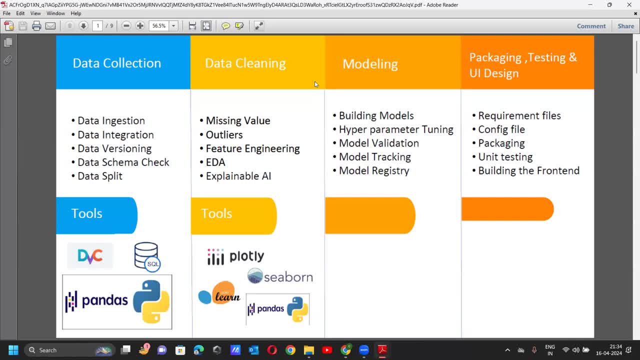 check, right, all data they cannot use for training, right. so security uh cybers at cyber attack security. this domain will have tremendous importance in future. so cyber security professionals, cloud- yes, cloud uh- will have a lot of importance. everything will move to cloud. so cloud specialist uh right um ai ops cloud specialist, cyber security uh- any. 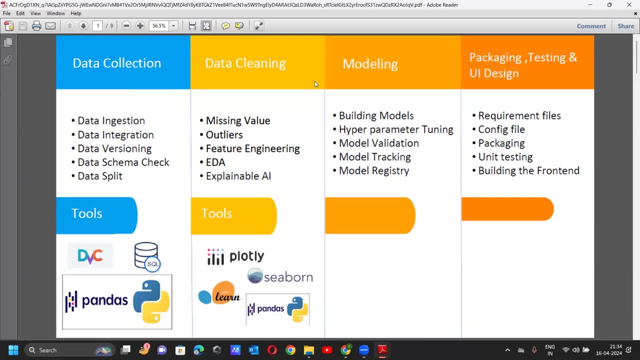 security related uh domain iot, like edge computing. these are the hardware side, right? um, uh people who will be building uh gpus and all that. so hardware side of it, this kind of role will evolve and which kind of role will go? software engineering role? it will not go. but, as i said, software engineering will be migrating to ai ops. 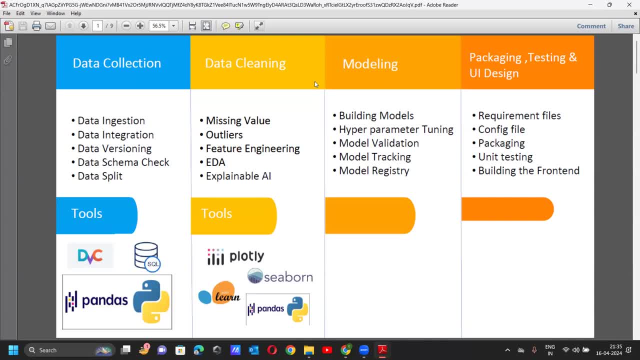 now we are learning ml of same thing- ai ops. so they will be building ai systems, they will be maintaining ai systems, uh and uh, yeah. so this is what i am thinking: uh, based on whatever the market situation. that's why you can see a lot of layoffs. many people are giving reason like economy is. 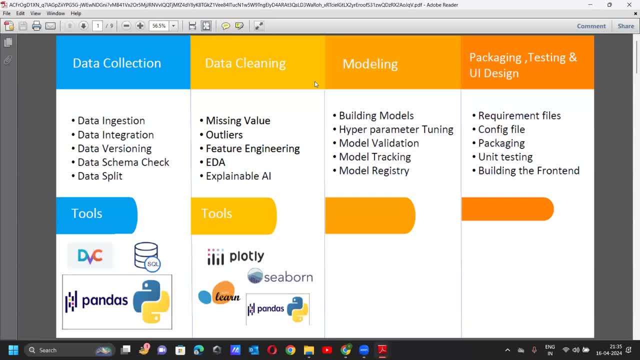 down, recession is there and all that. my prediction is: yes, economy is down, recession is there. everything is fine, but intentionally, companies are firing. i'll give you one example. let's take example of g general electric. it is a product-based company. they sell one jet engine. i mean they will get billions right and after covid aviation. 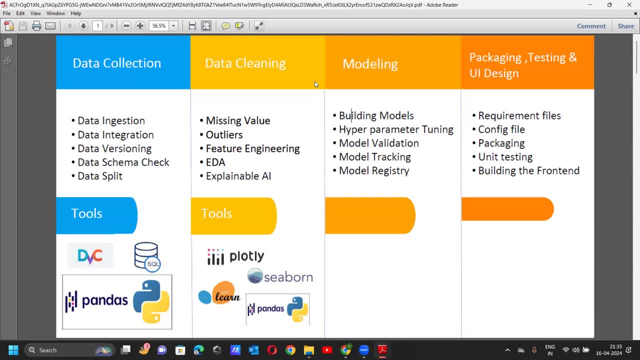 industry has been, uh, recovered, like anything. i did not find any reason to lay off, uh, their engineers, right, i mean, just because others are doing, they're doing. and why they're doing? because they're people mostly in product-based companies and in fact in service ways also, like. 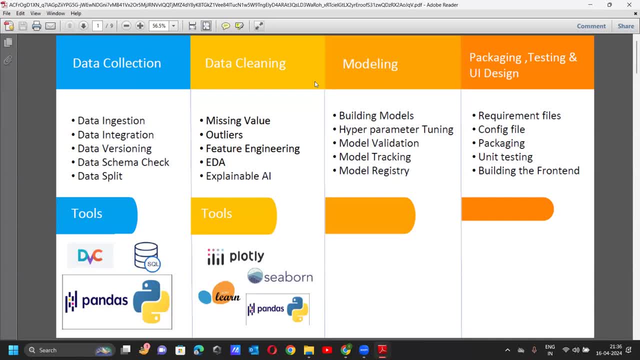 they're, they're in the company since years, five years, eight years, ten years, and they're not upgrading themselves and they're outdated, okay. and there are people, freshers, who like b take freshers and then maybe two, three year experience, five, four, five years. they are very much skilled. 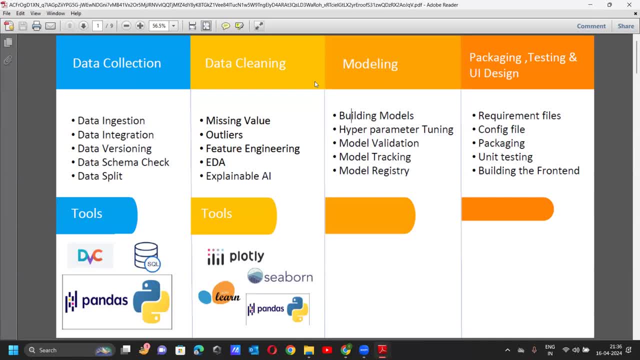 like they know generative ai. they know ai, they know the recent trends and less package and that's the reason of layoff. there's all things like economy recession. they're not upgrading themselves, are not the cause. skill, skilled resource- that's the i mean. they want to hire generative ai. 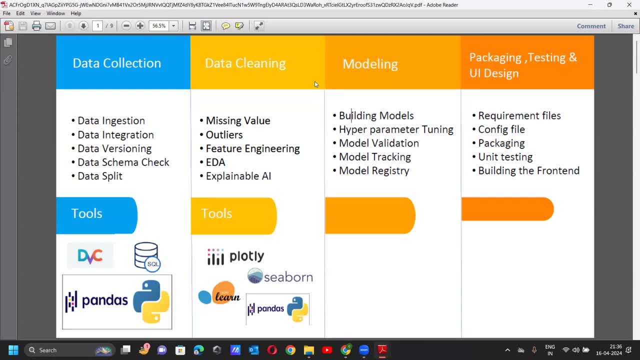 professionals they want to hire- ai related trending security, ai cloud. this professionals they want to hire. that's why they're letting go people who are old or maybe outdated. that's the only reason, and this trend will continue, even if the economy is good. this trend will continue. 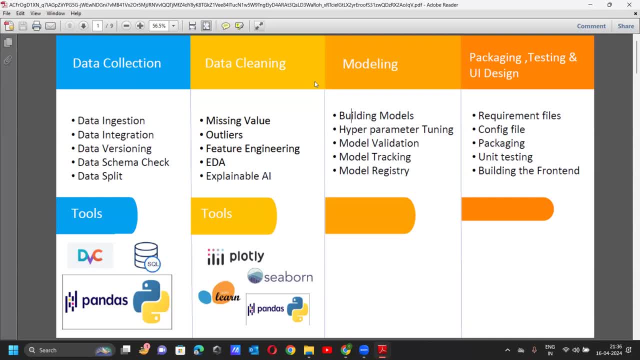 because really, if you are not upgrading company, don't need you right. and it will continue for two years, maybe four or five years, i don't know, but eventually uh it will be saturated, saturated means and in kilos how. how the uh placements were, like i, when i was in b tech, 350 student got placed. 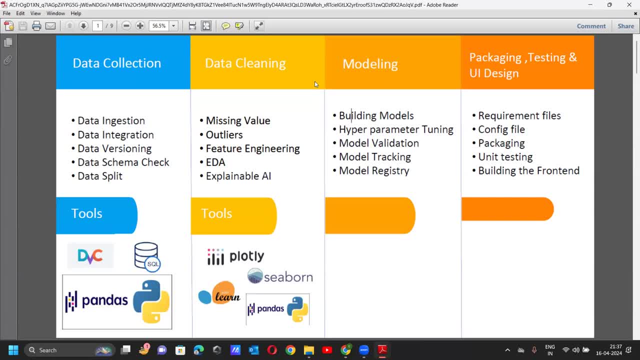 in tcs those kind of thing i i doubt it will happen in future. the headcount will definitely reduce. many of the things will be automated. so skilled people are required, not unskilled people, right? that is the main reason of layoff. it's not about economy. 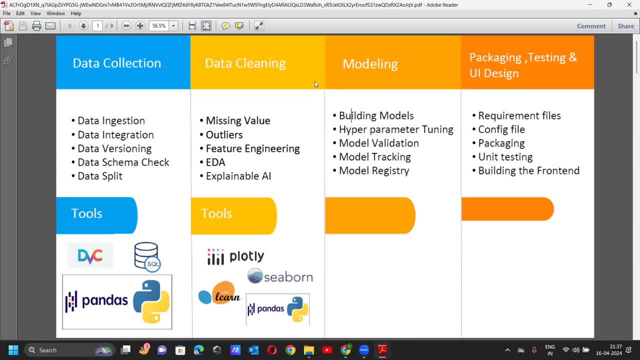 and anything, because i have seen companies who are growing like anything, but still they're laying off why they want to restructure their team. right, hire new people, let go old people, that's the new people means what? um ai, cyber security, cloud, iot, edge computing, all of this? 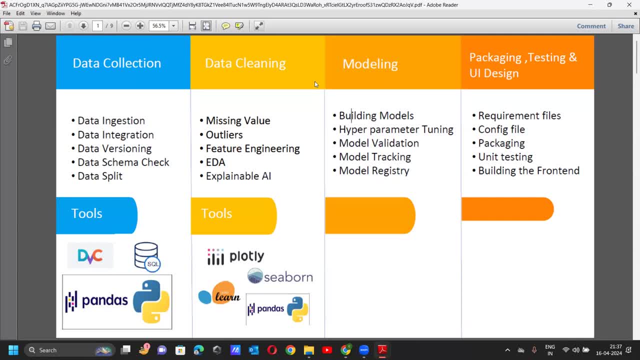 right. yeah, even in my company, they started layout, so that's why i wanted to quickly transition to you know some course which is in demand anyways, yeah, yeah, thanks for that. yeah, i mean, that is the case. i think, as i said, software engineering is going to be ai ops. i mean, now, that is where we 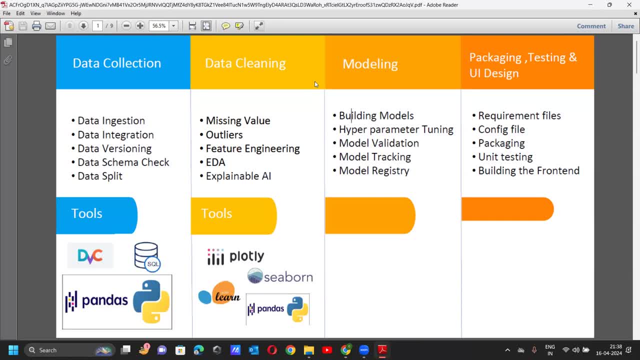 are going, not today, but eventually in four or five years, seven years. yeah, that's why they're pushing that generative ai gender dpi, so that you can build llm applications, uh, which are ai related, and you will maintain so. you will be a software engineer only, but you will be building your own. 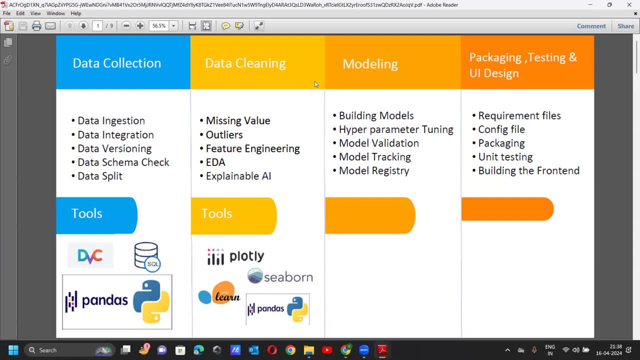 ai applications and maintaining it. okay, hi, ma'am, this is amit. yeah, am i audible? yes, i have almost close to 12 years of it experience and for the past i guess five, six years- i'm totally into business, making proposals, use cases, something like this, gtm activities. so is this uh feasible transition for me from a business side to into a data science? 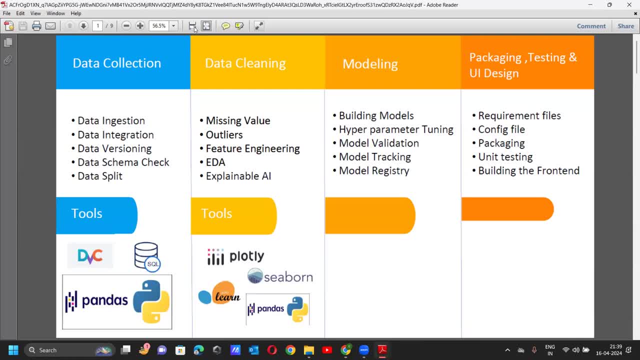 role. okay, so i will give you one thing: because you are in a leadership level or business level, uh, how you will generate ideas? because every product is ai right, and if you don't know ai, i mean you might not code, but if you work with a software engineer, you can do a lot of work and you might not know how to code. i mean, you might not code, but if you believe you'reicamente, you're good at programming and that's great, because that isgio in several content as well, in every involved gtm activities, how you generate ideas, because every product is ai showing the veterinary or social. 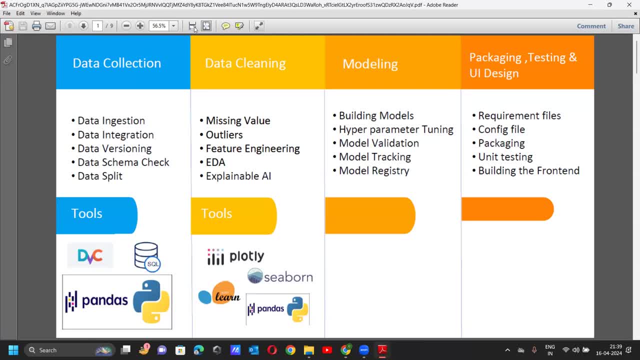 if you don't have at least intermediate level of knowledge, like what AI can do. I mean it is very difficult in today's world. I mean, what proposal you will create? right, Every proposal. AI should be there. That is the hype. 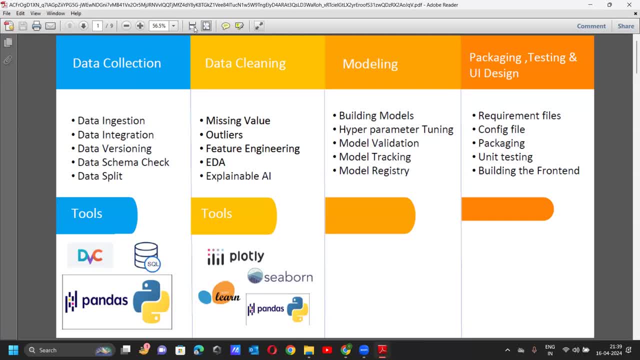 So if you, I mean if you want to generate ideas first, you need to know the industry right, What all things you can do, So then only ideas will come. It is not. idea generation is the most difficult task. Coding is easy. 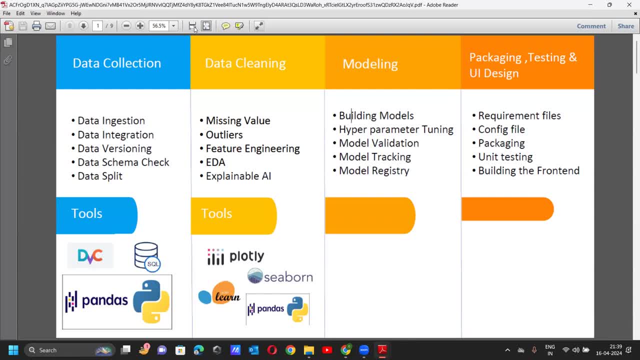 Somebody will tell you what to do and you will do it, But that You are finding that people are forcefully fitting Gen I or AI things to the real software right. I already told it, I think, long back. I think it's just a hype. 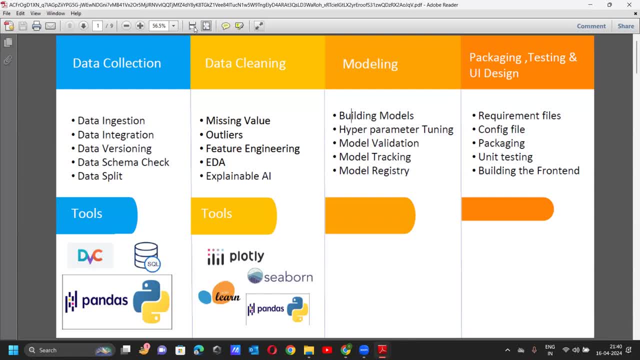 It will settle down in some time. I don't find Gen I applications are really- I told it right multiple times based on my experience- It is just a hype. So everyone is trying And if Gen I is, I mean, I cannot really tell anything. 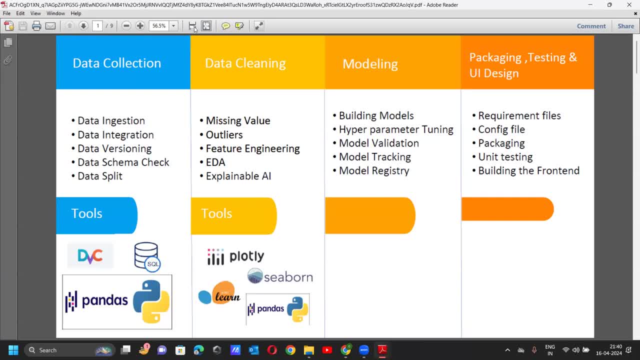 because the way the AI is going right- I mean if it is AGI, and I mean if you are getting really, really very advanced, even more advanced than what we have today, then there might be some possibility. But based on today's models it is very difficult. 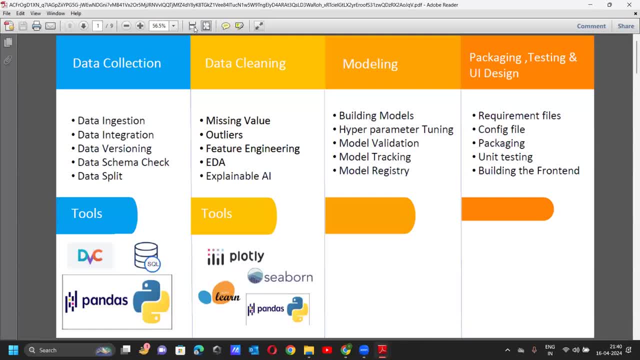 especially because of two problem three. problem Number one is Privacy. I mean data security, right. Second thing is: let's say you want to build something from scratch. Let's say you don't want to go for paid ones. 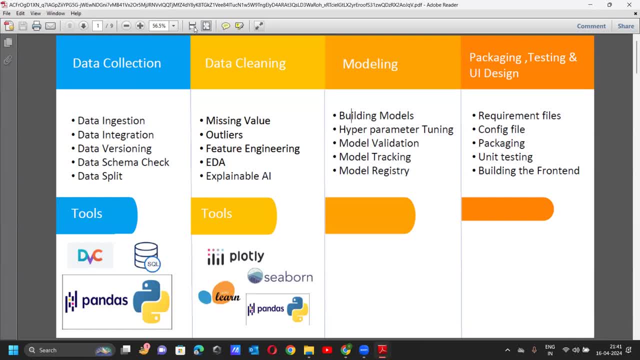 You want to build local LLM in your organization: lot of skilled resource which is not there right. That is also cost only, So you have to hire people. And the third thing is, I mean hallucinations, So I mean it might be good only for a. 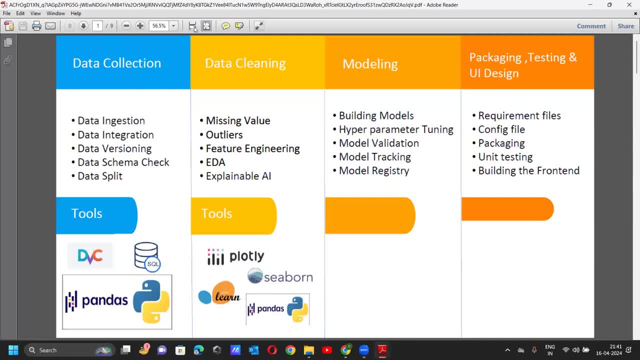 particular domain in the sense I told you right, Mostly good for text and image And in real time. we have organizations like healthcare and manufacturing. They may have some use case. but what about other domain Like mostly FinTech banking? they don't have much data on text. 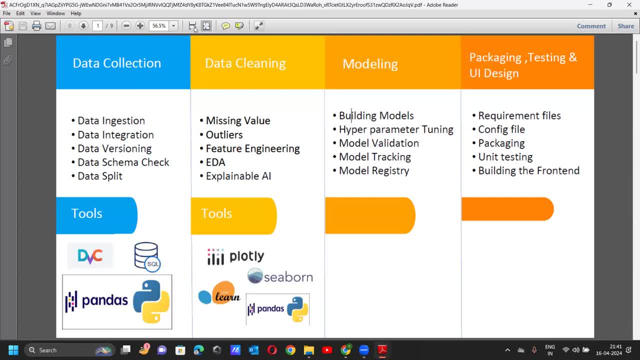 Mostly their data is semi-structured data. So I think for semi-structured data, I mean, if you ask me, traditional, the way I have written these things- the traditional ML, traditional deep deep learning Models, are better than LLMs in terms of cost, privacy, everything. 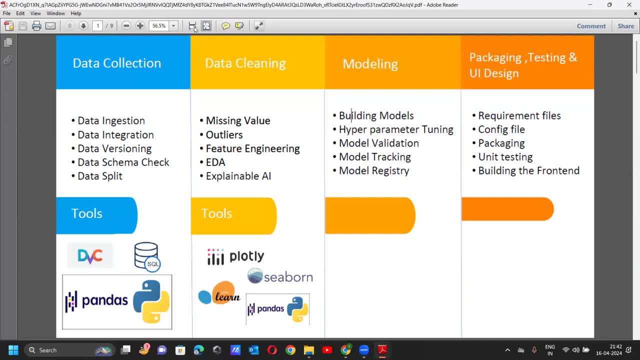 If you take that, those things into account. So I think it is so far it is people they themselves don't know, They just are trying to explore. but I mean, I think it is on only on POC level. I will say very rarely it will be successful out of a hundred, maybe 5%. 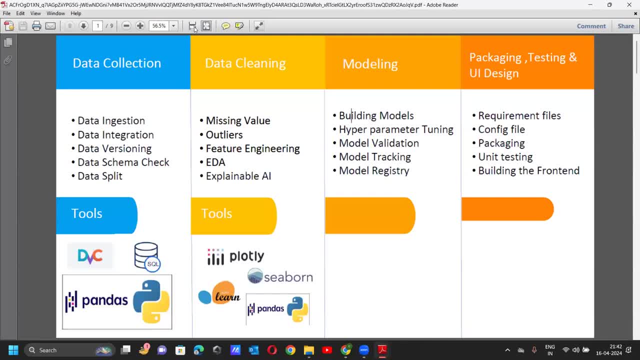 two, 3% will be successful, 18. 90% will be scrapped. but yeah, so it is a trend, So we are learning. Uh, yeah, So for my kind of experience, uh, is it good to learn this course or what? 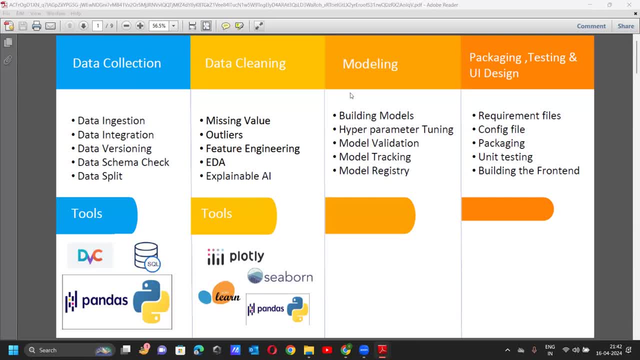 Go for the gen IE. one thing, Uh see, I think for you, if you want to generate, as I said, Jenny, Jenny is okay. So again, um, I don't know your domain, so if you can, let me know your. 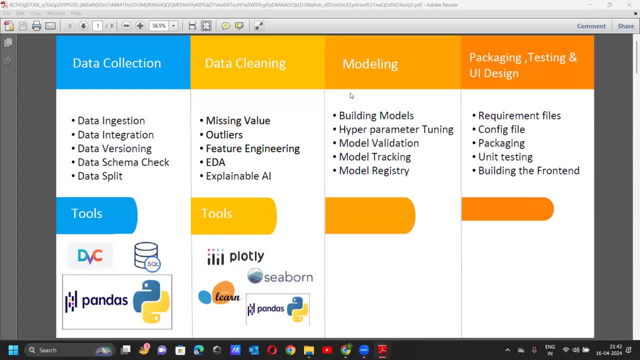 domain, Uh, background from which, Uh, my domain is like something complicated. Have you heard about IDC, Gartner, Forrester, for, uh, for yourself. One thing, Okay, I, I see you. you can understand from one point. 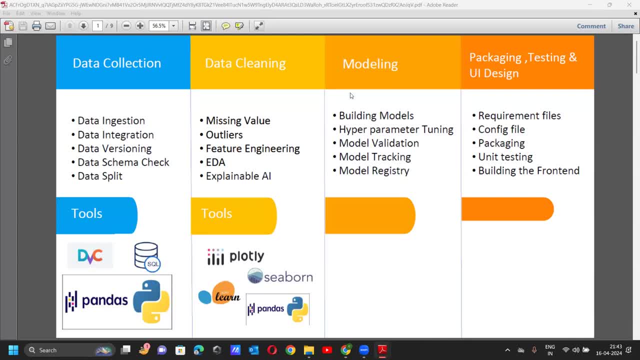 So you ask yourself one thing: So if your domain has a lot of text data, a lot of uh- video data, something like this, then Jenny, I course will be helpful for you and also you can Really build nice applications, because everything related to text can be. 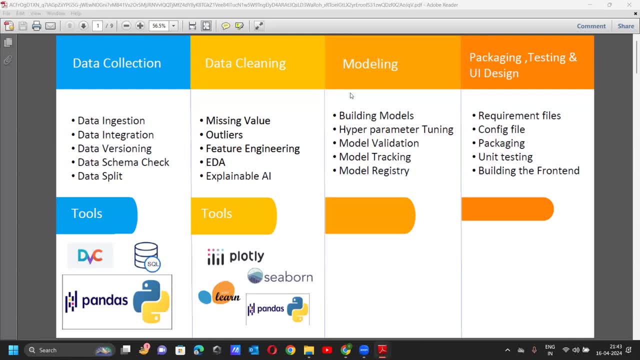 automated using elements. everything related to most of the things related to image can also be automated using LLM. So if you have dealing with unstructured data- uh, I think- Jenny, I course is definitely going to help you- means what you can really build production level. 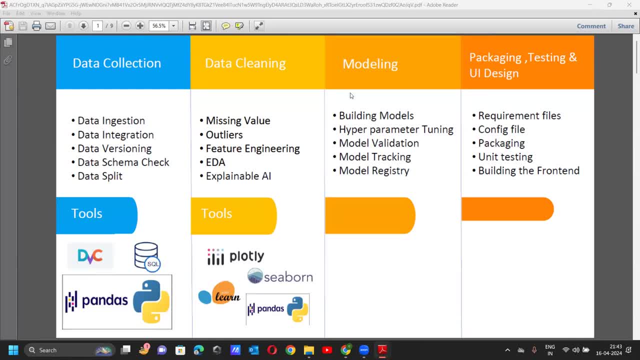 applications. but if you're dealing with Data, which is mostly, let's say, petabytes of data, let's say big data. I'll give you one example: When I was in BTM, I think, Uh, it is all about petabytes of data and uh, it's number data, right? 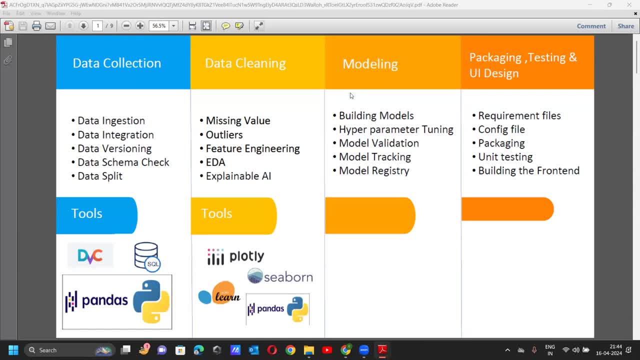 Mostly it is structure data, semi-structured data. So what LLM will do there? So hardly. what I can create is, I mean, uh, maybe our translator one language to other language. again, that is text. So that's what I'm saying. 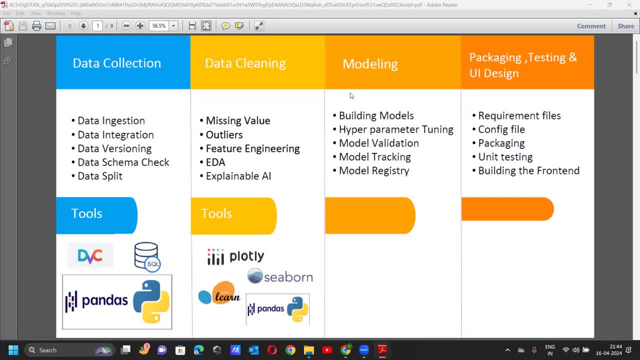 So I cannot generalize. based on your company background You can decide. obviously it will boost your CV. If you know, Jenny, I lot of calls, You will get interview. Why is it is very good, but application and real time usage wise depends where. 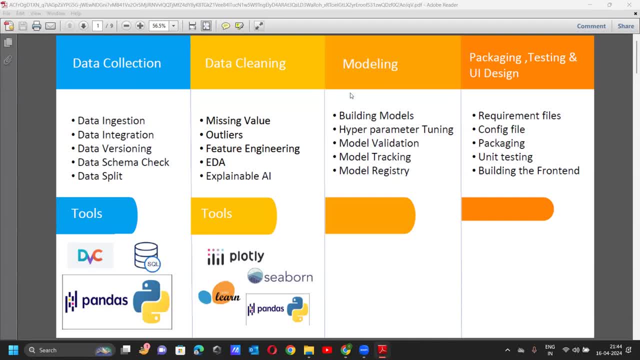 you are, and not every domain has Jenny application, not, I mean, you might not have any use case also. and uh, creating PDF documents searching and all that is a very common application, I think. uh, I mean domain, so yeah, sure. 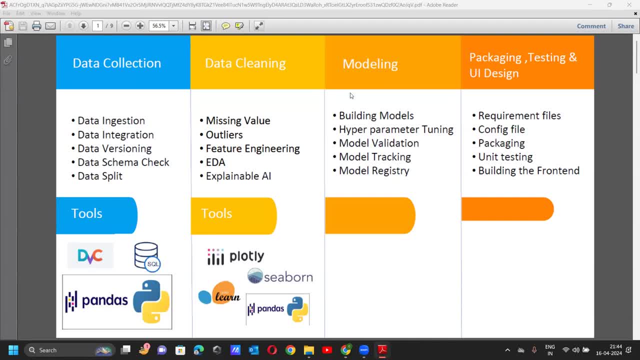 Thank you. Yeah, I said no. So it starts with lot of excitement and it ends with nowhere. So that's what is, Jenny In current situation. but, uh, there are certain areas, like if you are working with healthcare, Jenny, Jenny, I can do really great, great, great things. 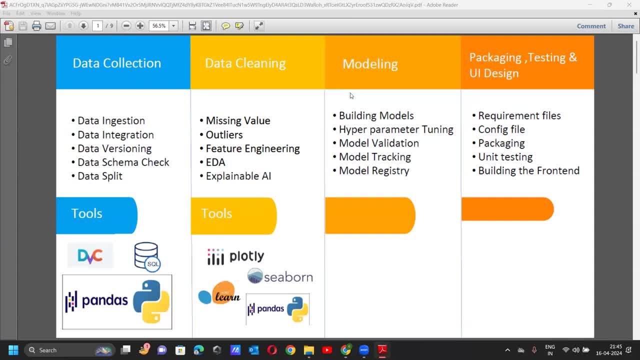 Uh text summarization: any uh named entity recognition translation. one language manager. language right Sentiment analysis. monthly multi-lingual sentiment analysis. and then uh uh, your uh image to uh text to image. image to text. uh audio data to text data conversion. 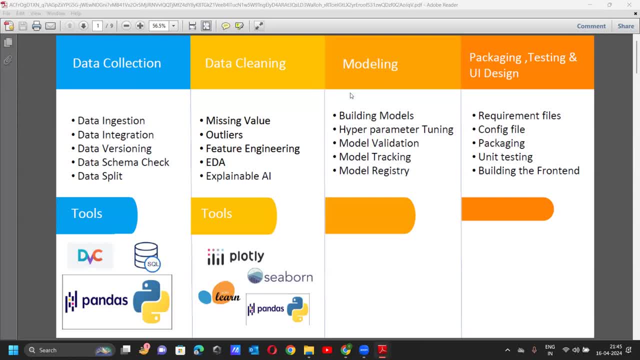 So all of these unstructured data if you are playing with. I'll give you one example. Let's say, in crack detection, uh, there are a lot of inspection happens in aviation. So, uh, wind turbines and all that So drone will go and collect footage, right? 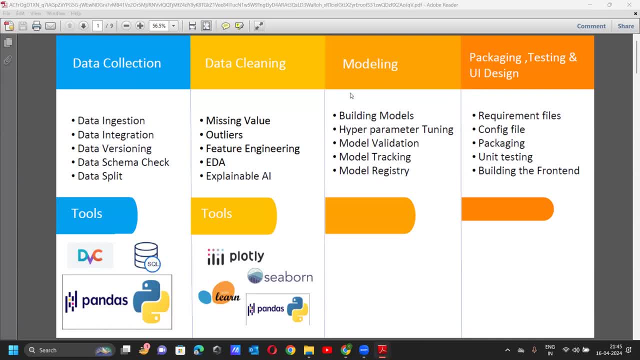 So that kind of application, Jenny, I can really be helpful. But if you're dealing with time series sensor data and uh uh PTM related data- like banking, mostly FinTech, I think- build simple application. why to make it super complicated, right? 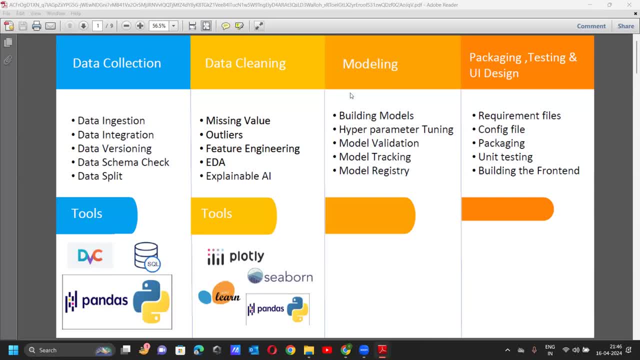 So, yeah, it depends, And you ask yourself what you want. You want to change into it- uh, sorry, into data science or ML ops. I think generatively, I will definitely help you in interview preparation. uh, because most of the companies- I don't know they have real use case or not. 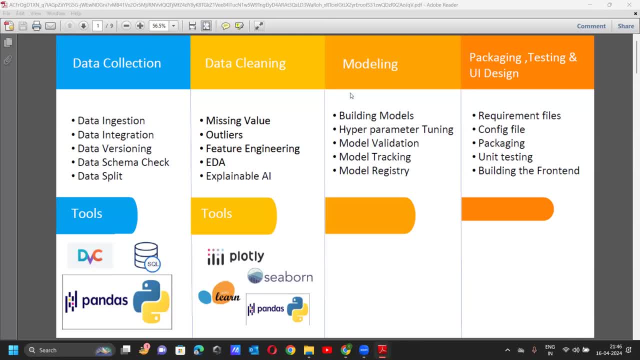 but they ask, at least in the interview. They definitely Right: Generative AI skill you should have. So I think in that way it is good. If your intention is already you, your organization has told you to upgrade yourself to build some application, then definitely the course will help you. 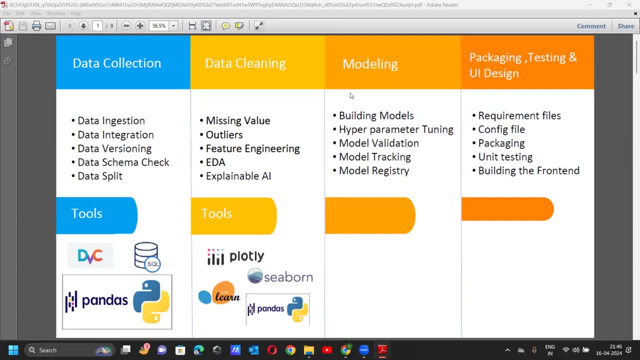 But if you think in your organization you don't have much unstructured data- mostly it is semi-structured structured data- I think, uh, Jenny, I you can learn for your knowledge. building real-time application might not be so good. 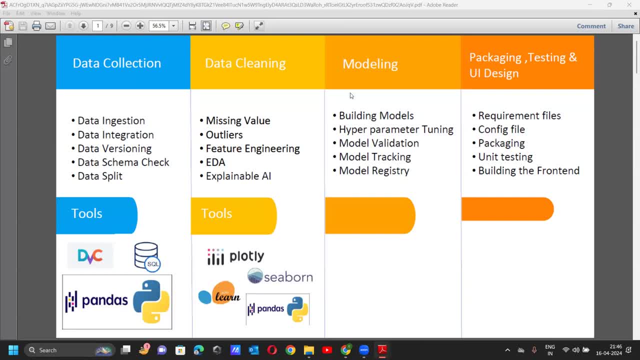 Can you hear me? Yeah, Yeah, Uh, this is Prudhvi. Uh, I have, I'm into QA domain. I have around six plus uh, SF experience in that. Um, but I work done um since beginning around five years I worked on um ML model. 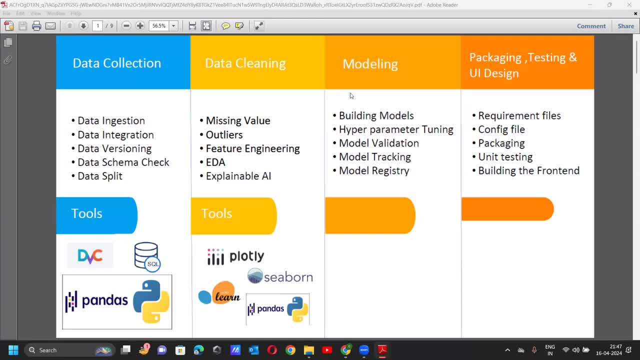 uh and IoT edge devices. I'm currently working on the ML ops uh project, Uh, okay. Uh, then, my role as a SDAT: um, I do testing those models and I use it to uh test the ML model accuracy and all. 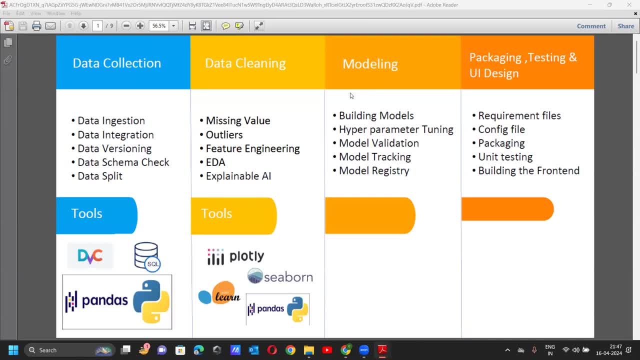 And currently I'm applying QA, uh traditional QA method, to implement. I mean uh to test the models or the flow. Uh, actually, I want to uh join this course because I want to uh test it better. 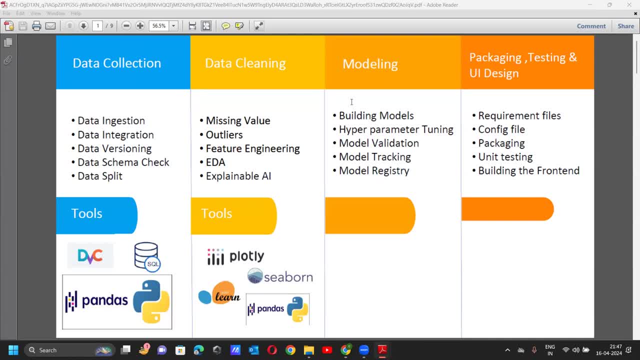 If I, if I know this, I know the flow exactly. And uh, yeah, I have two questions for you. Like, uh, I'm getting calls as a AML tester. Is there a score? Is there a score for uh AML tester? or uh, do you say? 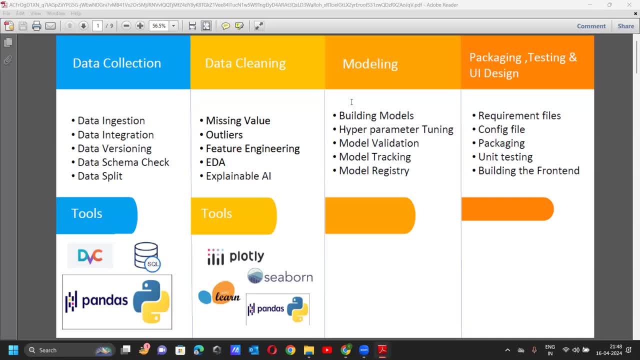 I will tell you one thing: Okay, Any kind of testing is already included in development. So, whether it is software testing or a ML model testing, I think this is something called validation, which is already a part of modeling. And also We do unit testing, five test and all that. 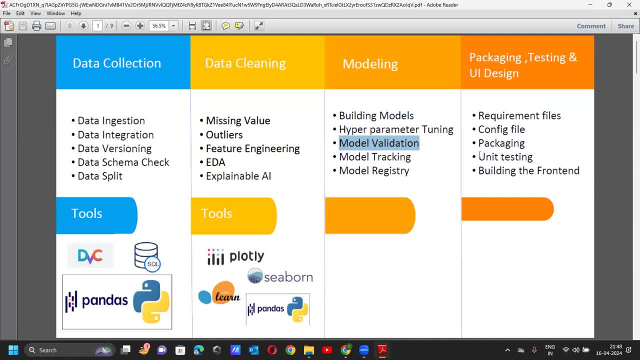 But having said that, mostly we validate our model. This comes later. I mean, if you don't include this also, it is not wrong. I mean it's not a blunder in ML, but this validation is a blunder If you skip this. validation can be done only by the person who has built the model. 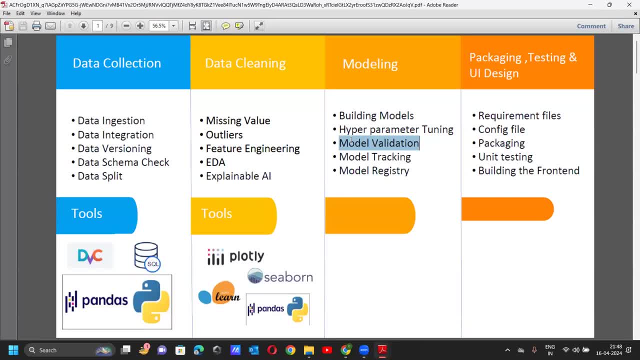 I mean one person will build and one person will validate. No, that is not how- something we do in ML, because we have certain way of validating. Again, it will vary from project to project. when you are dealing with the classification, your validation will be. 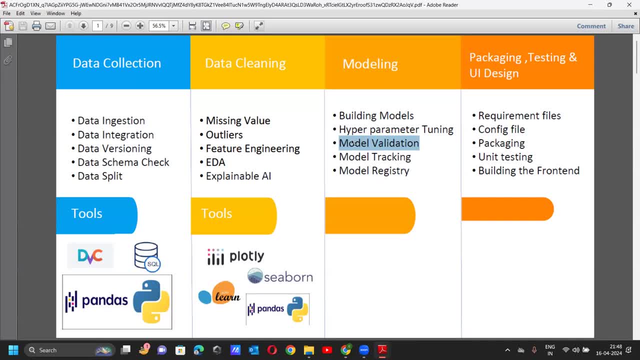 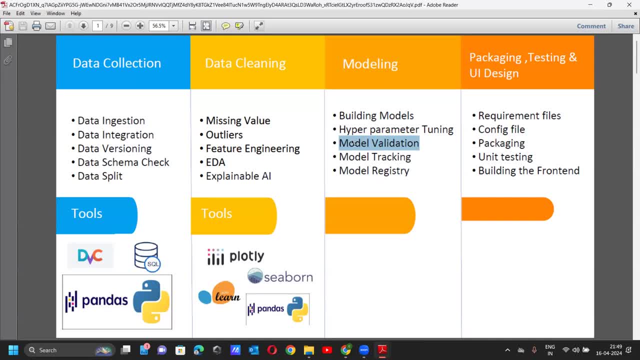 If it is a regression, MSC, So we have different metric right. If it is a customer related problem, we divide into cohort And then. so what I mean to tell you: the person who has built the model has to validate. 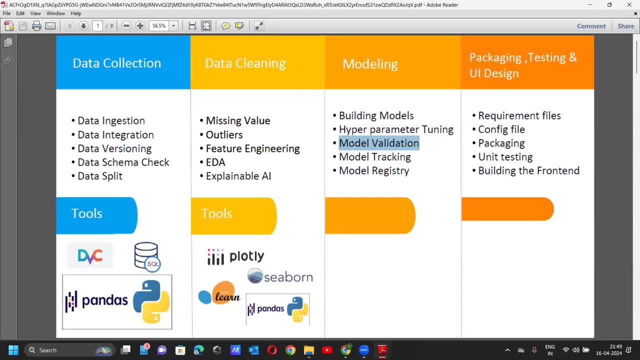 And uh, it was never. it was. I am hearing this term for the first time like ML tester. It was never in. I mean, It was never a role like validation is always a part of modeling. but yes, prior to charge, a pity. 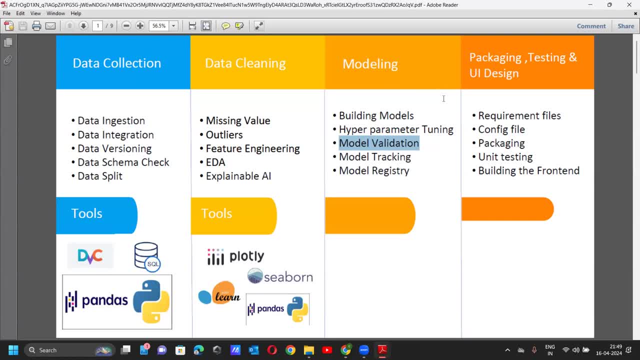 I mean, if you go back two, three years back, The modeling was the task of a data scientist. uh packaging, testing, UI design, uh deployment mostly web, web app. uh like development team, like DevOps, uh the Tom DevOps, software engineers and data engineers come by. 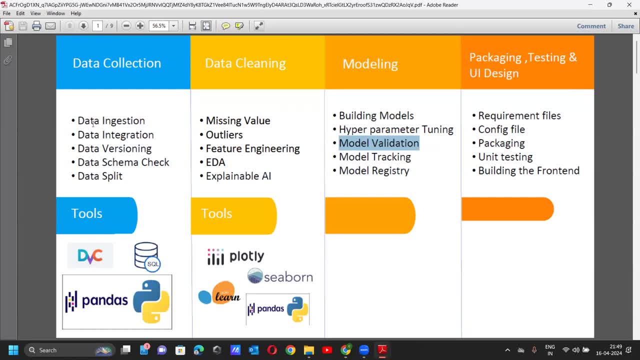 In fact, this collection also, uh, in real time collection, is not so easy. right Data, And in fact today also this collection part has been taken care by. they have their own tool. It's not so simple. uh, in real time. uh, you have a lot of things. 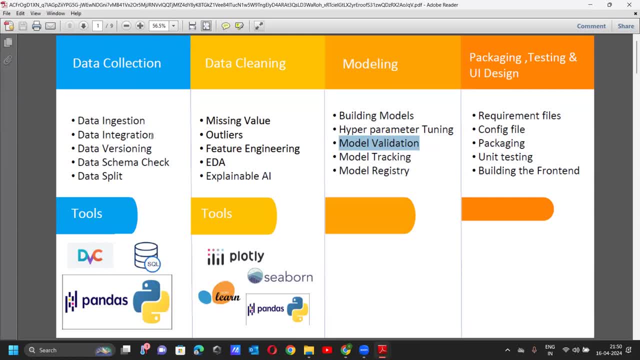 So airflow they will be using, snowflake They will be using, So that those are mostly data engineer tasks. um, as a data scientist, your major task is cleaning, modeling, packaging and then deploying. That is what your task. monitoring also, but ETL and then um, so I mean um you you got. 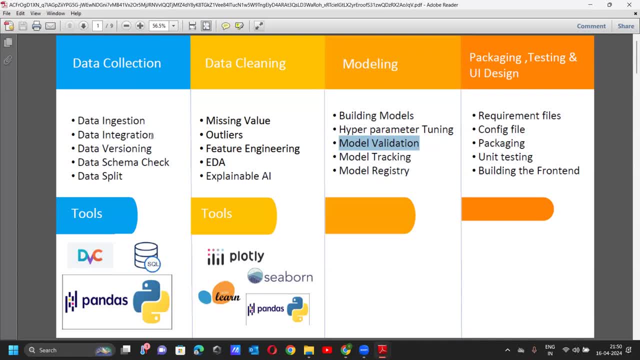 My point. So before there were, there were a team who will be supporting a product. product means everything: front end, backend. So front end means web app development team. They will be creating the front end flask applications and all that react flask HTML. They will be exporting that and also CI CD pipeline. 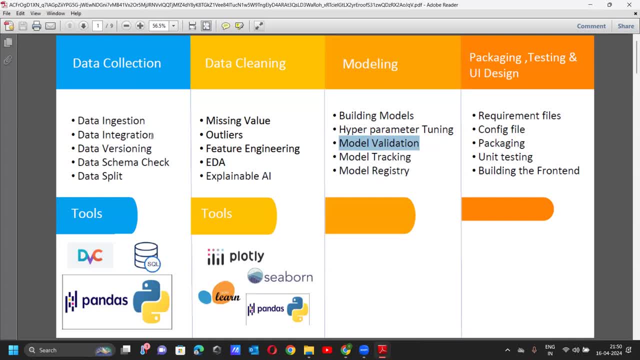 All of these things they will take care. data engineering team job is ETL. They will provide you data in a particular format. Their task is ingestion, integration, versioning, schema check- everything They will do. data reconciling: They will do the installation. 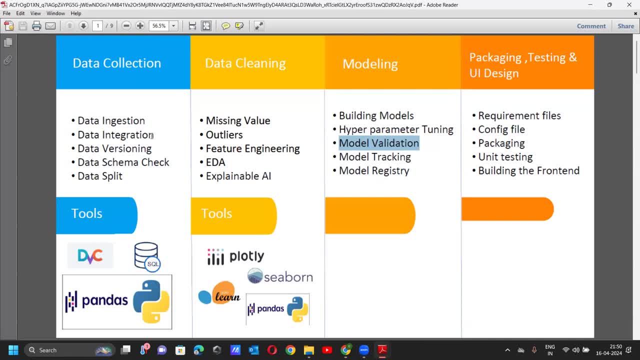 Your task is: collect the data, build a model, deploy the model. Right, So, um. but because coding is already automated, companies are expecting full stack, Um, a person who at least can build a simple app, a front end, and deploy- uh. this kind of roles are evolving. 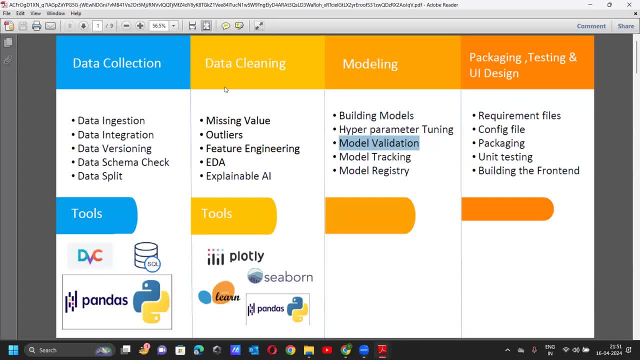 So, answer to answer to your question: definitely, everyone should take this course, for sure, If you want to Come to AI, AI, AI, AI, AI. This is the foundation course and the generative AI is definitely it's a hype, but that's the next level course. 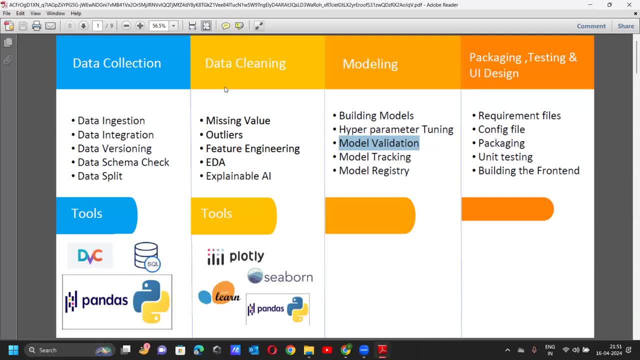 Um, if your company is pushing, you are in a hurry. So maybe you can take the generative AI course first and then maybe you can learn yourself. but uh, honestly speaking, without this course you will not be able to understand the machine learning part. 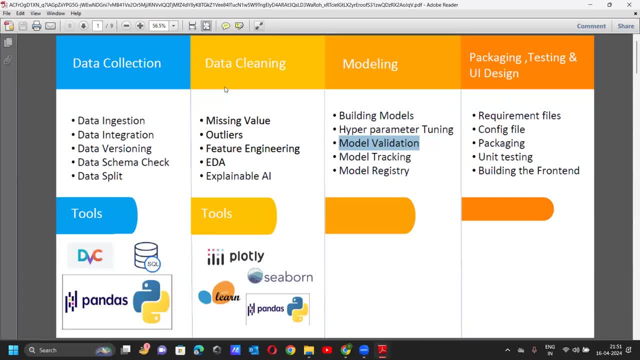 Deep learning. Anyway, I will cover in the Jenny I all the unstructured thing we will cover in Jenny I. but most of the use cases in Real time are still semi-structured and structured, So those kinds of thing you will not be able to understand if you have skipped this course. Jenny is the next level, but this is the foundation level. 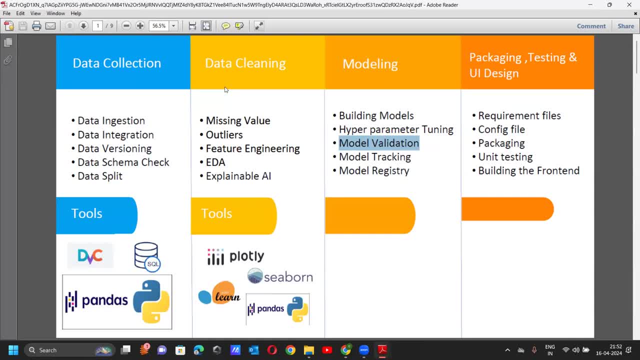 Again, it depends. Uh, you are working in healthcare and all the data is unstructured, So maybe you can skip this course and you can go ahead with the Jenny Right. So I think you've got an idea, So I think um. 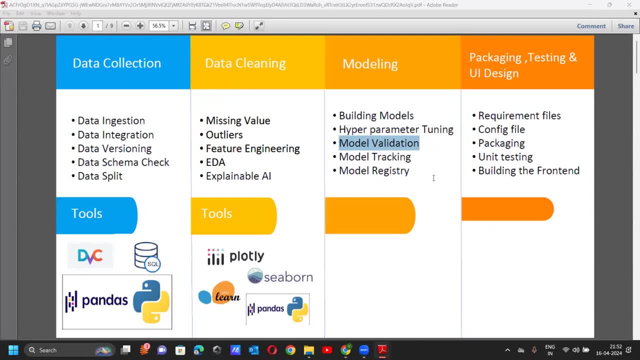 I'm. building model and training model are the same. Exactly Same building model, training model, same building. No, no, I mean same thing: training. So you will understand. about the training, validation and test, We split our data into three parts that we will do here when we get the data right. 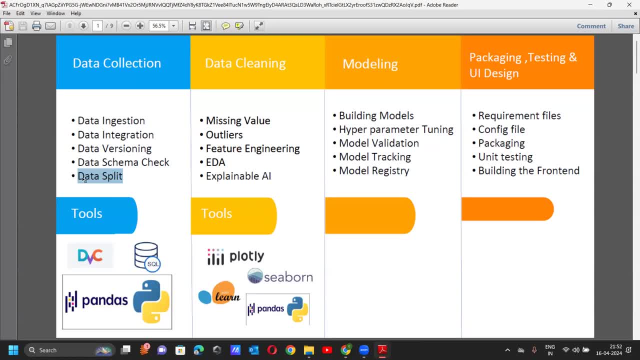 We will split it into training, validation and testing. So yeah, So I think building models means training Only training models, Yeah And uh. one more question was data cleaning. Does that depend on the algorithm that we are planning to use or independent? 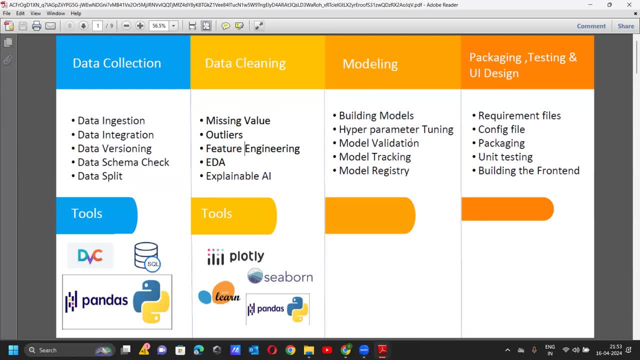 No, no, it is different. Modeling is different, Like we have different set of algorithms for modeling. We have set of algorithms for the cleaning, like outliers. we have isolation forest. We have a lot of algorithms for feature selection. We have exit boost, uh. so feature selection and outliers EDA. 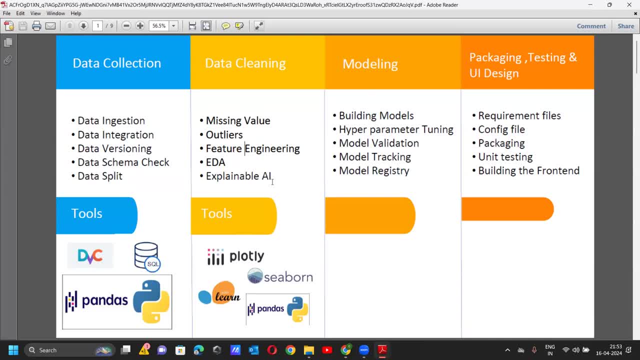 We are going to use- Plotly explainably, I, we are going to use a tool called SAP, SAP Lee, Uh, yeah, but like which algorithm to use? that decision comes in which stage? in data collection stage or in data cleaning stage? data collection: 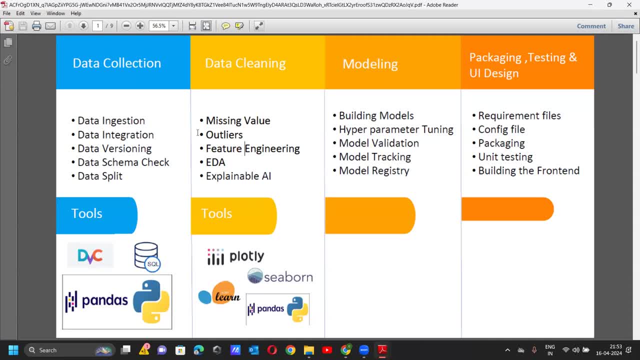 There is no algorithm, It's just Python script You will write, but data cleaning and modeling, you will be using algorithm and validation, So don't worry. So once you start the project, you You will be knowing right. I have read one line. one more confusing term is data engineering and ML engineering. 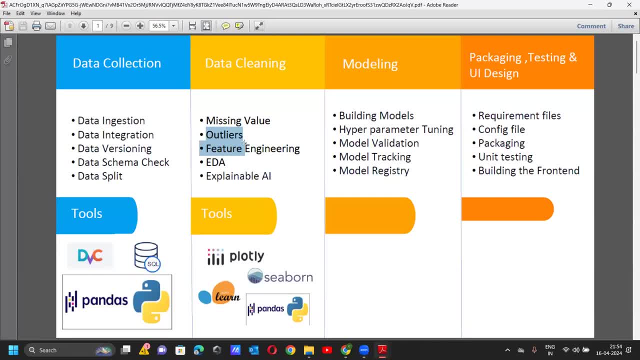 What is the difference in these two, The ML engineer and data engineer? many companies, they treat them as equal, Many companies that treat them as different. It really very confusing, uh, to me also, Right, And to everyone also. it's not only you because, uh, data engineering was a very separate role. 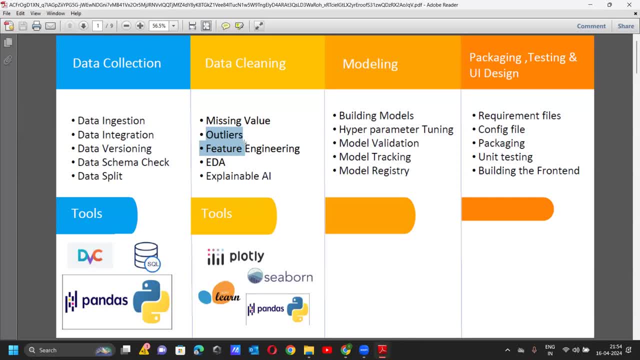 But after 2022, when the ML ops engineer engineering role it, it came to market. many of the. it is really confusing So many of the data scientists and data engineer. they migrated to ML ops because it's a both, two in one. 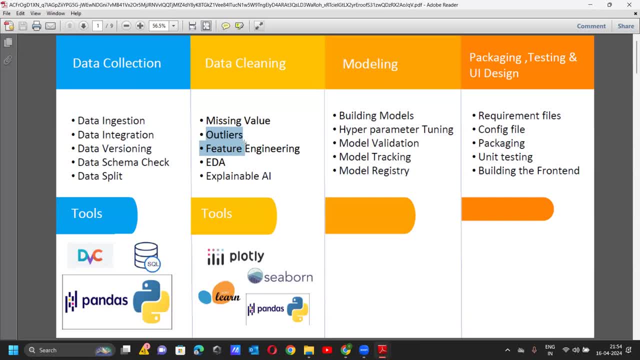 Right Ops. data engineering is. data engineer is very strong at ML, data scientist is strong at, so it's a two in one kind of role. It's a full stack role. So if you ask me the main Major difference, I mean again, it differs. it differs from company to company, but major. 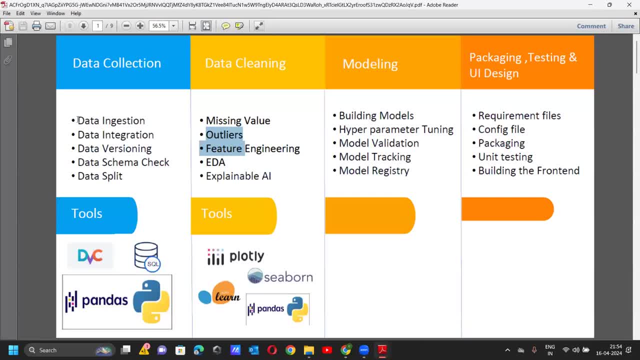 difference is this part. So a person who is a data engineer, they should be very good at cloud. not one cloud, maybe one, two cloud, two cloud at least. uh. AWS, Azure, AWS, GCP, any two cloud uh expert. 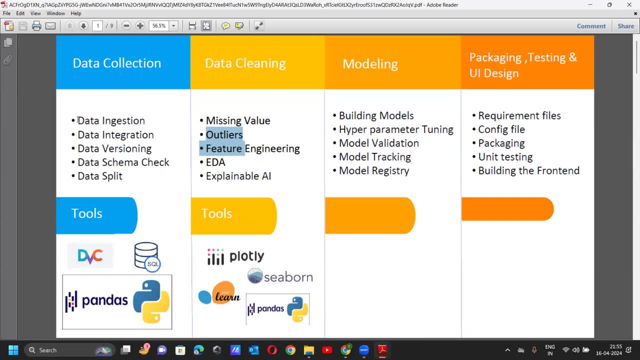 means what they should be knowing. all this like not only ML, the administrative kind of things, the how to create IM user, how to give Access to which kind of user. if I give you full access, you can do whatever you want. 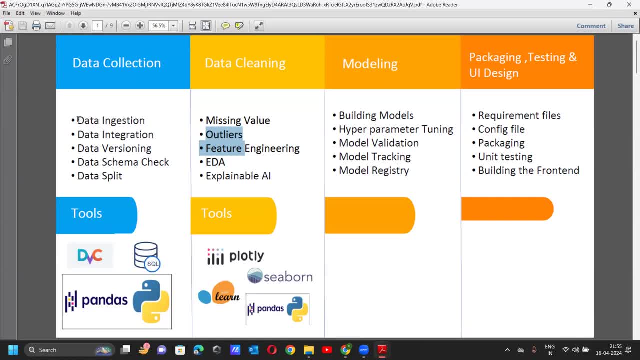 to do Right. So I need to give correct permission to correct tree team. So it's a very uh, uh, like it's a great task, confusing, complicated task, in real time right Budgeting they. they need to decide the architecture, the, the complete data platform. 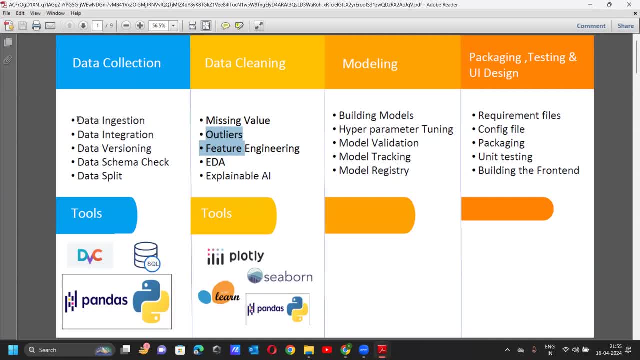 They will decide. So, data engineer, data architect: these are the people who are very expert in cloud. They know everything. We are not that expert, We Just use cloud for deploying models, but they are the people who will build the cloud platform. 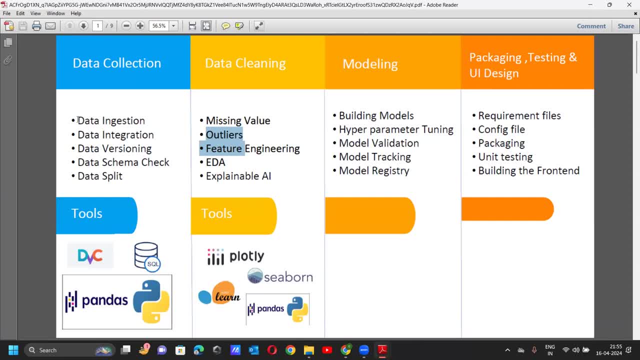 for your organization. Not only that, they will give proper access to everyone. along with that, They're very good at big data, so they can handle any variety of data, any streaming. They will be knowing Kafka, Scala, uh, Java C, sorry, Python. 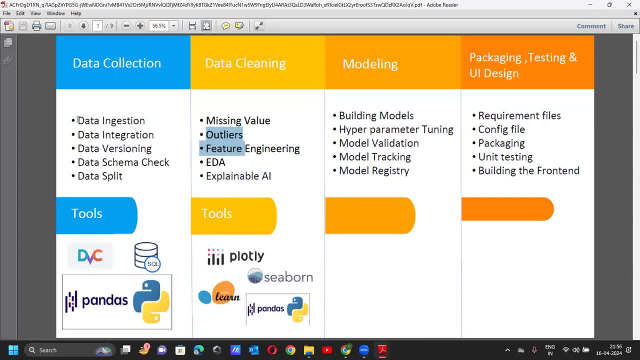 They will be knowing Apache, air flows, no Fleck. So there are a lot of tools with respect to data ingestion and uh, they will be knowing this. um, BBC for data version Control, get to get up. uh and uh, they'll be doing a lot of databases: uh, redshift, AWS, redshift, and then SQL MongoDB, because data can be in any format. SQL, no SQL. 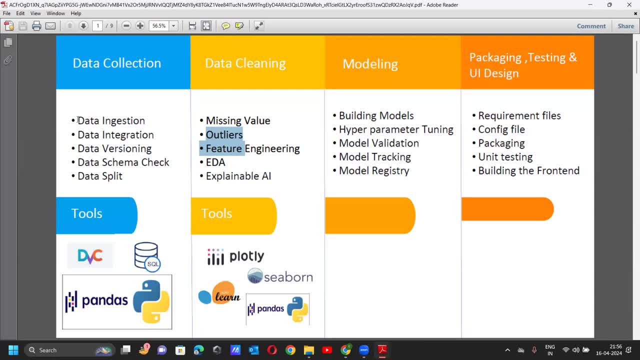 Right, And uh, they are the people who will do ETL extraction, transformation and load. Uh, they, they are very good at data lake, creating data lakes. everything they will take care of, So you no need to worry about the data platform. uh thing right. 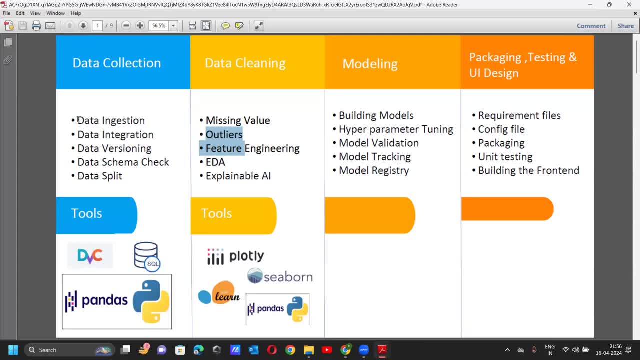 They will take care of it, They will maintain it, They'll create it, They'll maintain it, They'll give access everything. So that is Data engineer. Now, ML engineer is mostly responsible for uh, uh again. um, as I said, this role is really confusing. 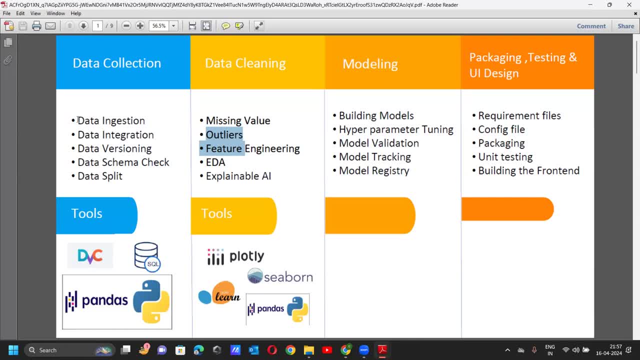 Most of the time the responsibility of ML engineer is from. I have seen companies. mostly they're looking: okay, Modeling, maybe data scientists can do, but packaging onwards, everything they need to take care means what they are very good at: packaging modeling and uh uh versioning and then 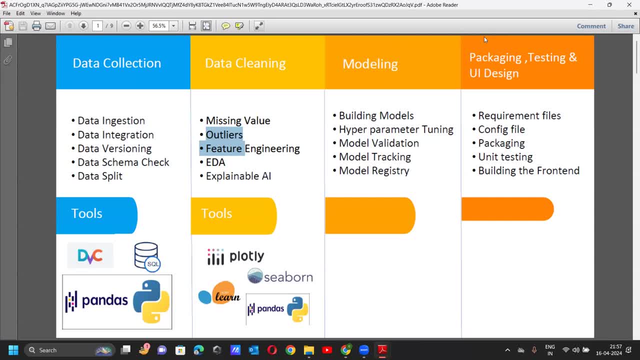 And then Taking it to uh production environments, staging and then trying in the production server, deploying, maintaining all of those things Right Along with uh this, this entire flow that you're looking is mostly ML, ML, engineer task. 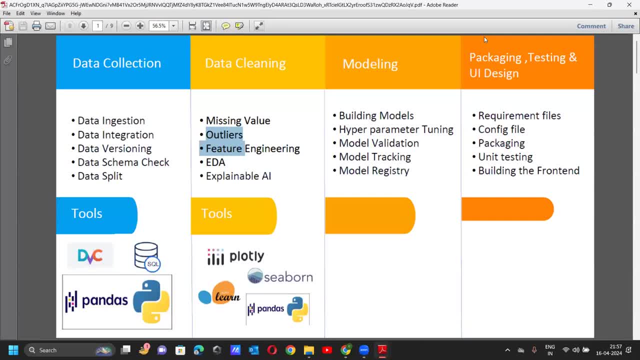 Right, Yeah, Yes, Yes, Not So ML ops. And so this ML engineer now what they have done. they have in the JD, they have written everything. So if you look at the ML engineer, everything, Yeah, Yeah. 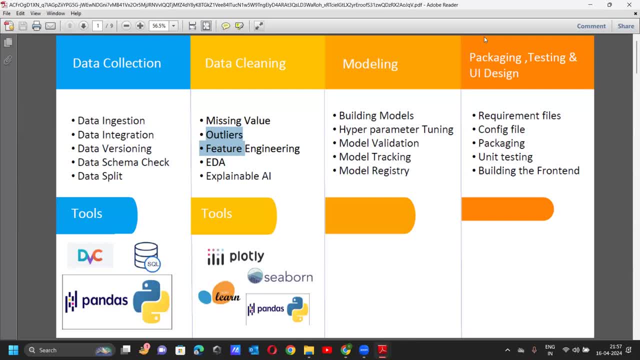 have written: data engineer, data scientist- everything they have combined. they should know airflow, they should know snowflake, they should know big data. they should know this, that, this, that don't worry about it. 70, 80 percent- if it is matching means you are a good fit, never it. 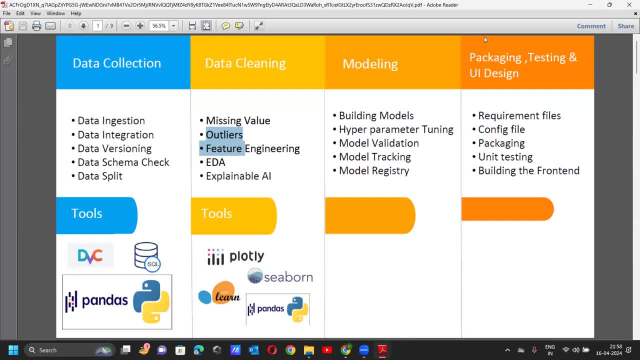 will be 100 match. even my profile will also be not 100 match. none of the person can match 100, so 60- 70 matching means you can apply for those roles, so it's a very good role. um, you got it right. so there are different roles: data architect, data engineer. these are a different. mostly they will 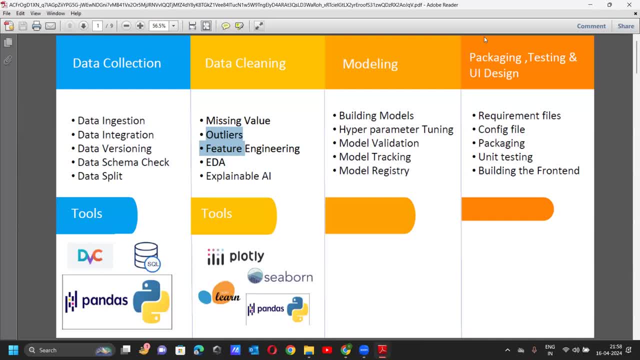 be building the platforms for the company right ml engineer. they are responsible for uh, maintaining the ml models in in real-time production environment. right, and i think data scientist role also is going to be converted to ml ops. there might not be any. there will be research role where people will be building llms, new innovation, but 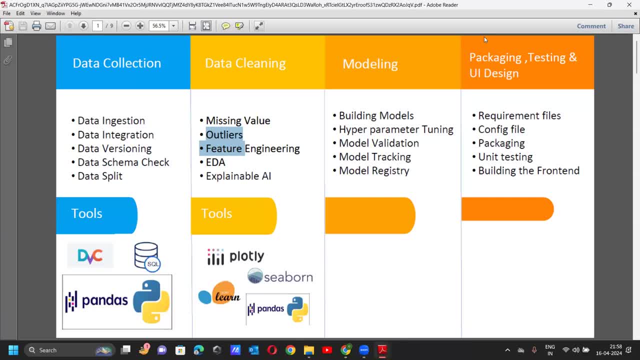 otherwise everyone will be engineer. only riveting um engineer means cleaning, modeling, deploying all in one, because modeling you are not doing, char gpt will do modeling for you. once you have done the script easily, i mean coding- is already automated. so ml engineer will do everything and researcher will create new, new ai systems, ai models. that's a different line, research and 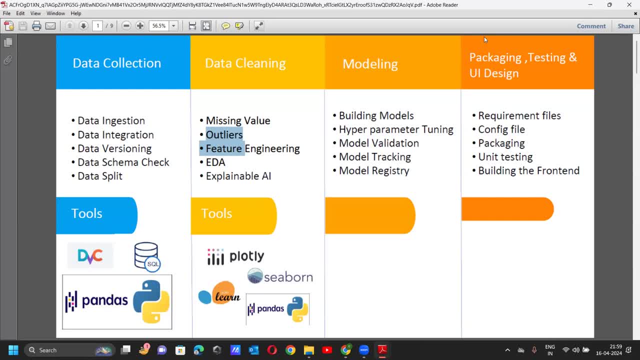 development. so i think you got the idea. it's really confusing, uh, but i think, um, there is a very thin difference, thin line difference. yeah, i think i i can take last one or two question. i'm getting late, yeah, yeah, okay. so, coming to ml ops, can you please let me know what are the topics that you are going to? 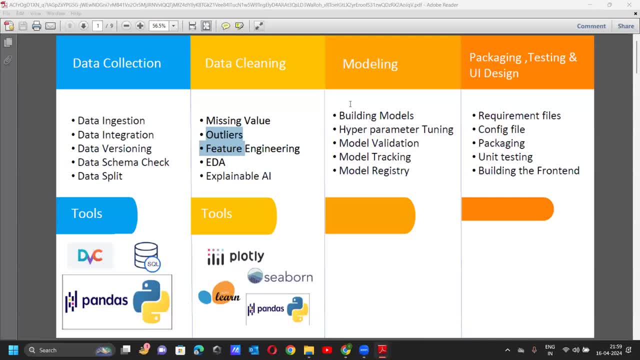 cover on these ml ops, like you are going to cover ml ops for containers and edge devices. all these topics are going to cover on that, this training. i will be covering dvc. if you are asking tools right only with respect to tool, then dvc ml flow. 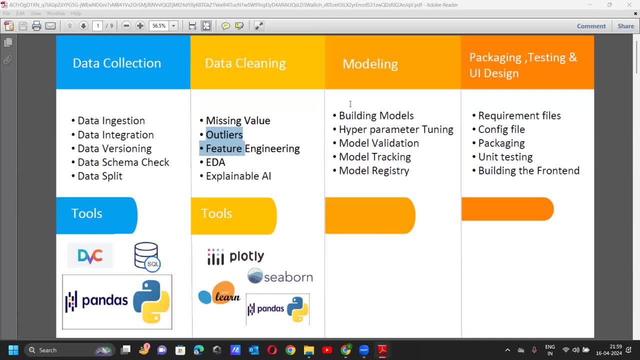 sage maker. um, obviously, for modeling, we'll be learning sk, learn right uh, and the machine learning algorithms and uh pi test for testing right uh, followed by dockerization. so we'll be using ecr, elastic container registry, for dockerization and uh. these are the major tools and then streamlit for creating front-end plotly. 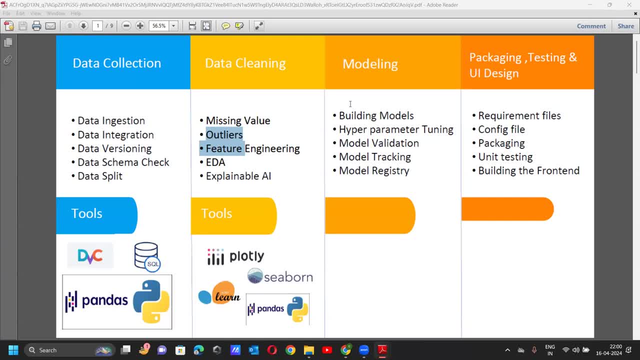 uh, pandas for data manipulation, right, so it's all around it. yeah, so everything is going to cover under ml ops, right? yes, yes, so don't worry, it is not an ops course, it is ml ops. so i will give equal importance to ml and then ops. so first, second and third, these three pillars will be: 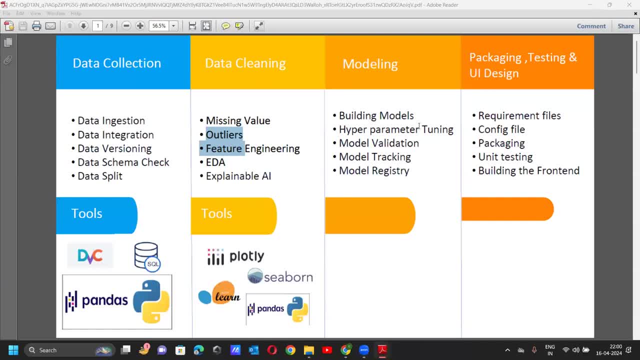 it is totally on data science part, right, cleaning, modeling is all data science. from fourth pillar onwards it is ops: packaging, testing, ui, design, deployment. so fourth pillar onwards it is ops first, second, third is especially second and third is uh, like the the data science part. you can say, or 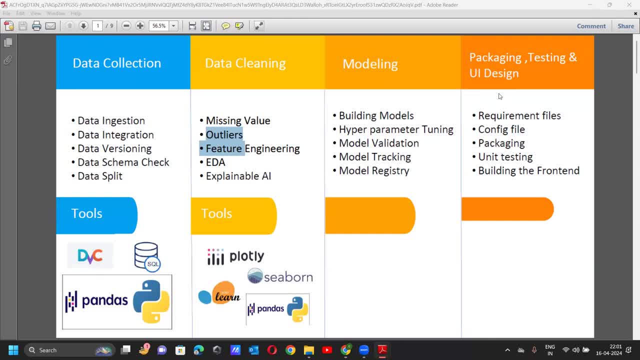 ml part, so you'll be cleaning your data and building model and validating model right. so we'll do these things very, very uh, you know, in a very, very deep uh way. we will understand not only machine learning. we'll also use keras for a deep learning project and in the gen ai uh also, we will be discussing a lot more. it's totally on unstructured 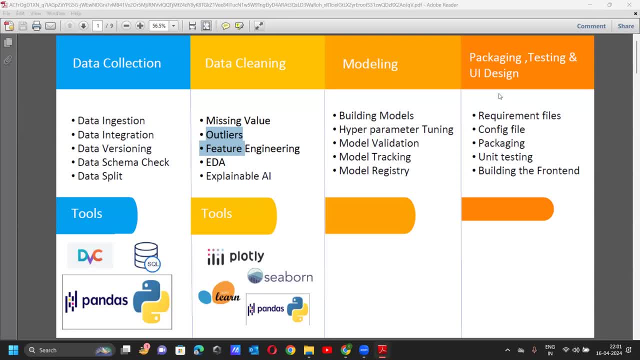 data. so all the projects that we will do is on image and text data, right, okay, okay. so i think, uh, just give me some time. i think by tomorrow you will get the complete syllabus, i will finish this three project and i can share it with you, so everything will be clear. 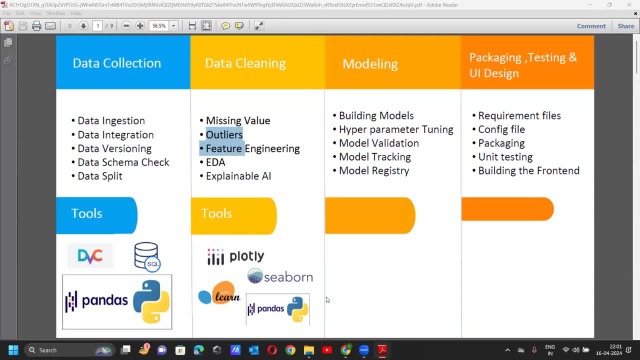 in fact, in every step, what all tools i'm going to use. also, i will write for modeling, what else tools, packaging and ui design testing- what all tools. so you will be getting clarity, topics and the tools right. is there any whatsapp created for this session next monday? we will create. 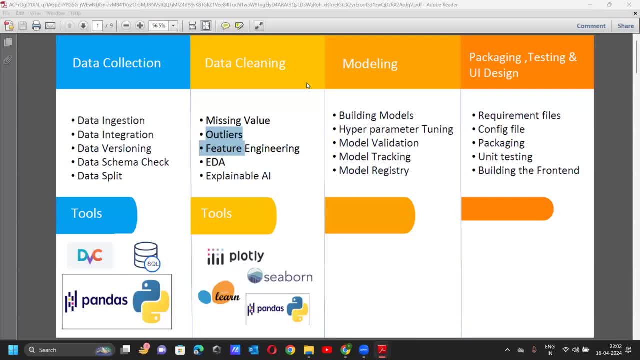 i think this friday the bridge, the link will be reached right and we'll inform the batch. so monday i will share the whatsapp link. you can join. thank you hi. yeah, one more class is there, eight to nine. so what is the timing for this one? this is nine to ten and one more is there morning 7: 30.. 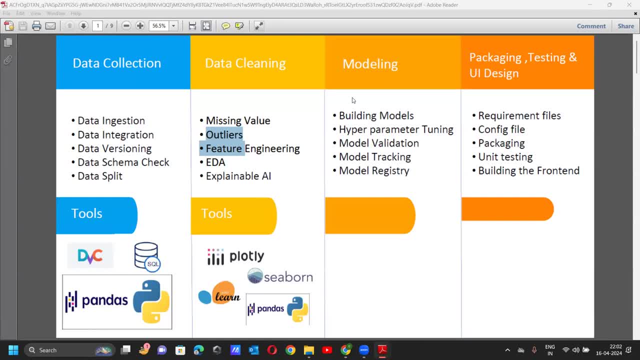 uh, okay, but uh time is uh nine to ten only uh evening. and one more is there: 7, 30 to 8, 30.. 7, 30 to 8: 30: yes, morning. nine is the six now, yes, nine is fixed. yeah, nine to ten, yeah, thanks, so that was my class. 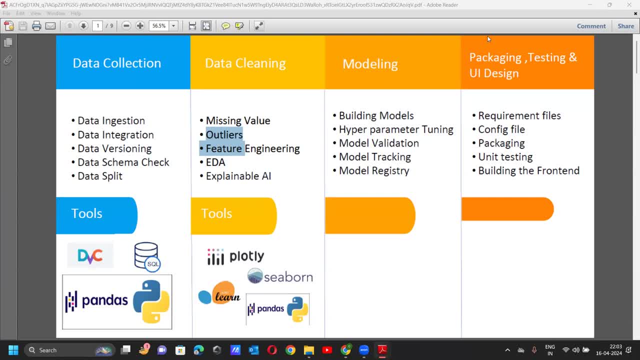 so tomorrow onwards we will start with installation. uh, very simple things. we will discuss about vs code and other thing and git, github repository setup and everything but uh, i will just show you the content, uh, maybe 10-15 minutes, and we'll start with the content. 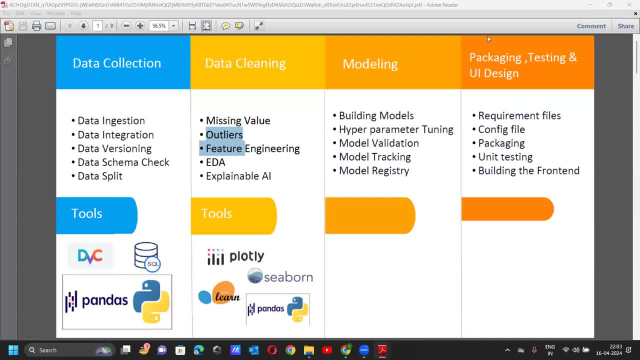 in the sense software installation part. once the class is over 30 minutes only, we will see and then next 15 minutes. if you have any question, you can ask, and this week i will give a quick review or summary on the core python part. next week onwards we will be starting with pandas, right? 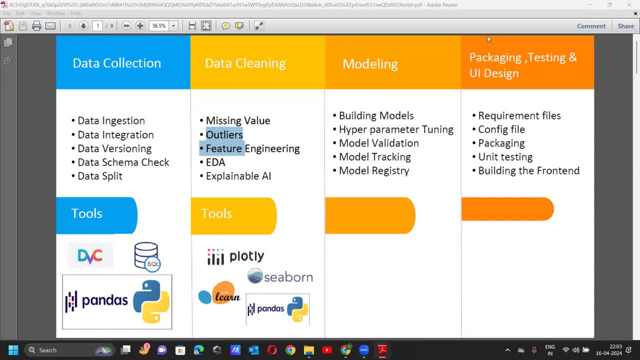 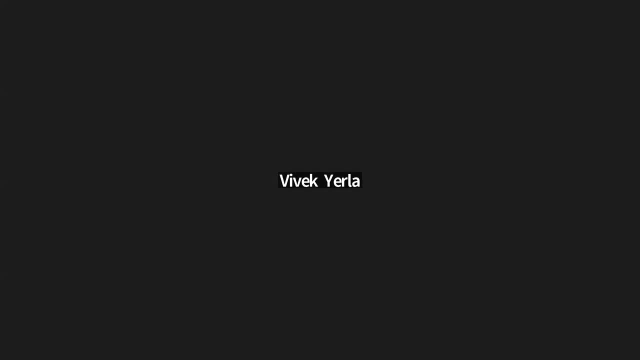 um, okay, okay, thank you everyone. thank you, ma'am, thank you, thank you, thank you.